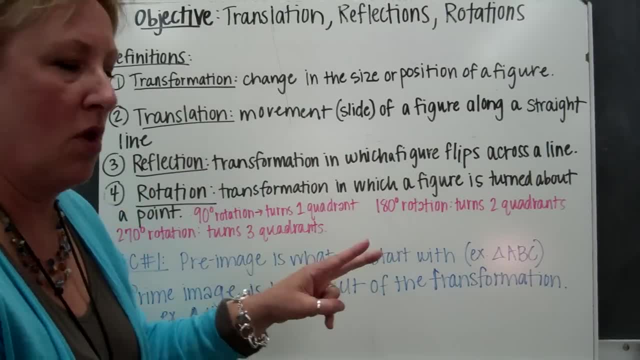 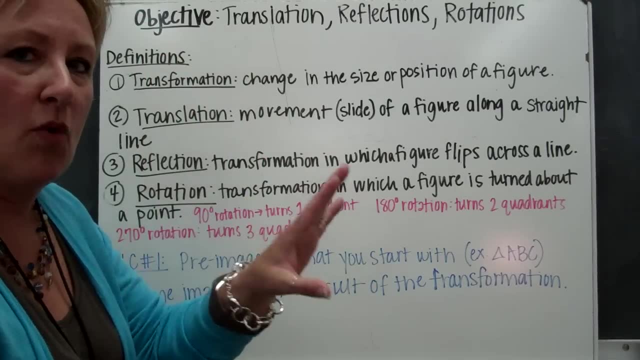 quadrant plane And a 180 rotation turns it two quadrants. 270 degrees will rotate it to the third quadrant And if I do it, 360, I have got it right back to the place of where I started from. Very important concept number three. 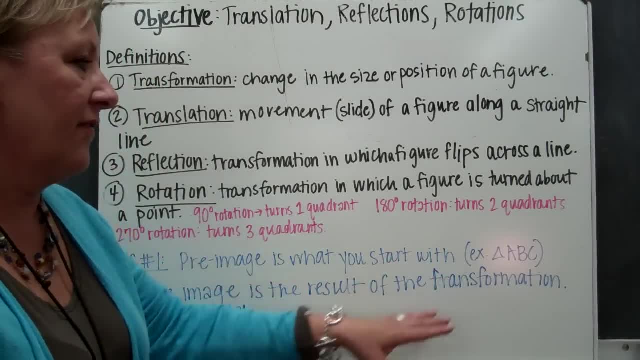 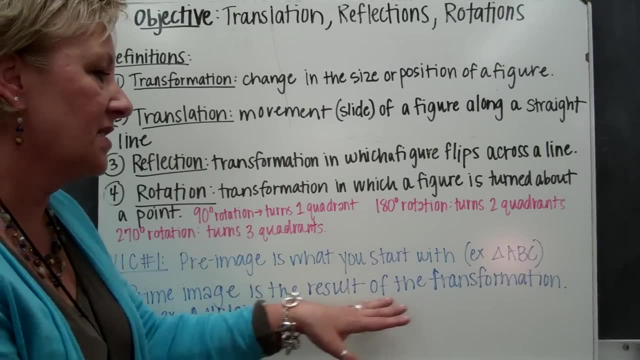 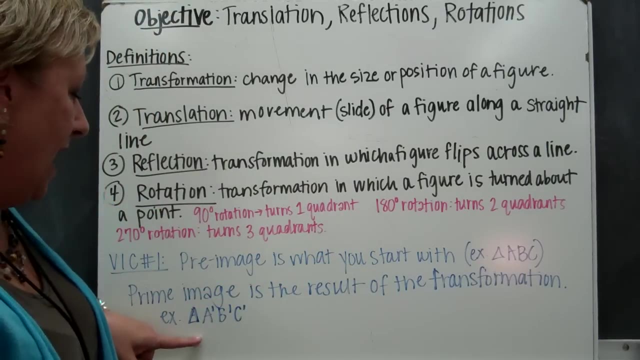 Number one pre-image is what you start with. For example, if I have a triangle ABC, I'm going to have a prime image and it is going to result of a transformation. So if I've got triangle, ABC is my original pre-image. my prime image is going to be looked at with. 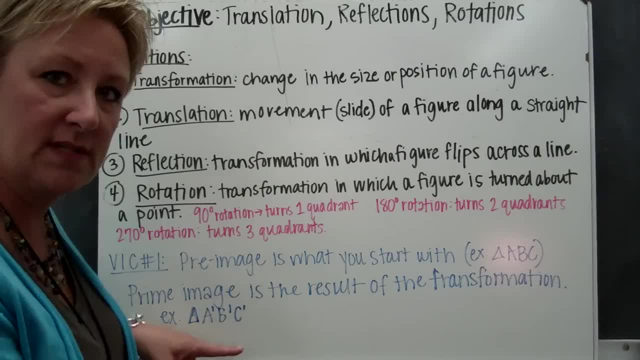 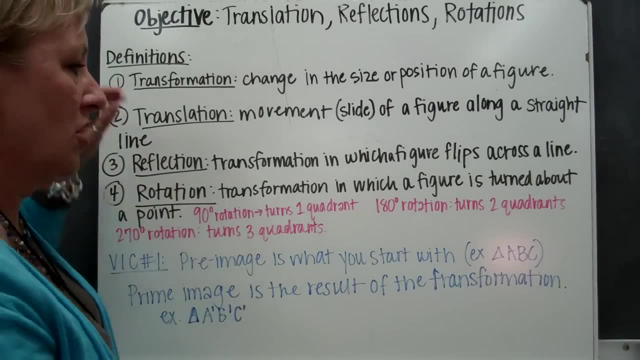 an A triangle: A hash mark, B hash mark, C hash mark. If there's one more than one hash mark there, it means that it has been changed twice. The very important concept number two: A translation slides the figure left to right. 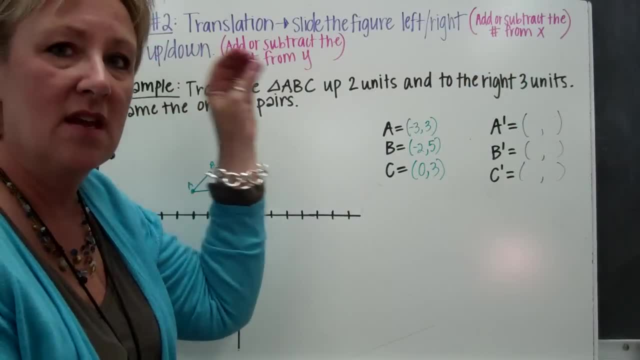 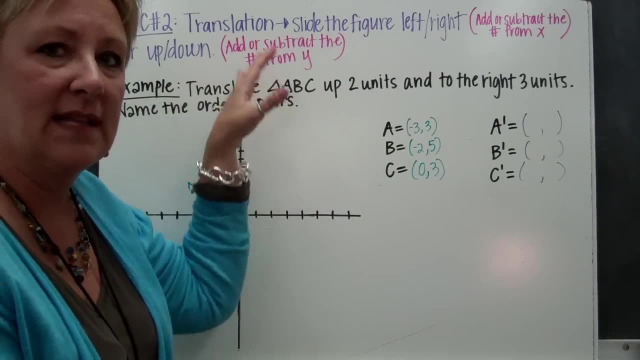 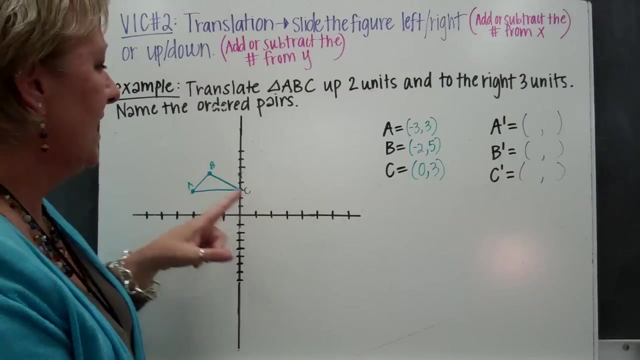 If it goes left to right, you're going to add or subtract that number from the X value in the coordinate point. If it goes up or down, you're going to add or subtract the number from the Y axis or from the Y coordinate point. For example, if I translate A, Y and 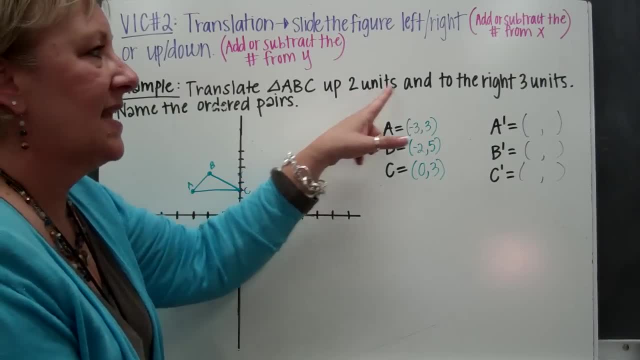 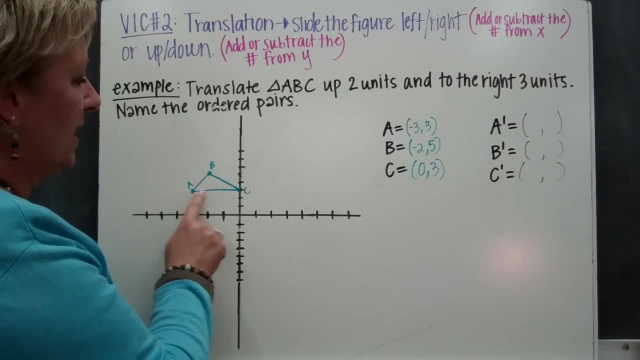 B triangle ABC, up two units and to the right three units. I've got to name the ordered pairs. I already know that A is negative three and negative two, B is going to be negative two and this is going to be one, two, three, four, five, five. C is going to be zero because 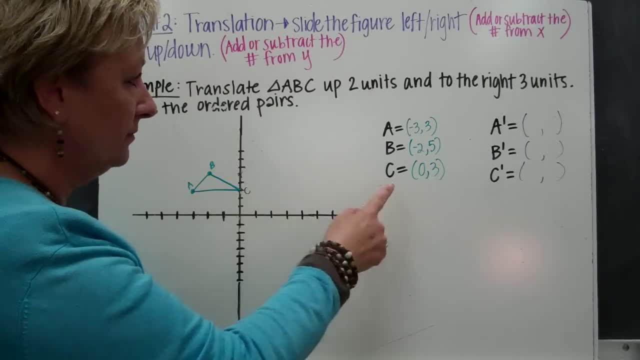 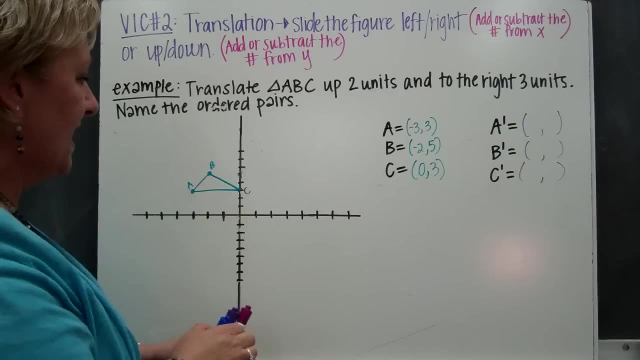 I don't move it left to right on the X axis and three. So if I want to change it by the, by going up 2 and over to the right 3, if I go take A and go to the right 3, it's going to go over 1,, 2, 3 on the y-axis. 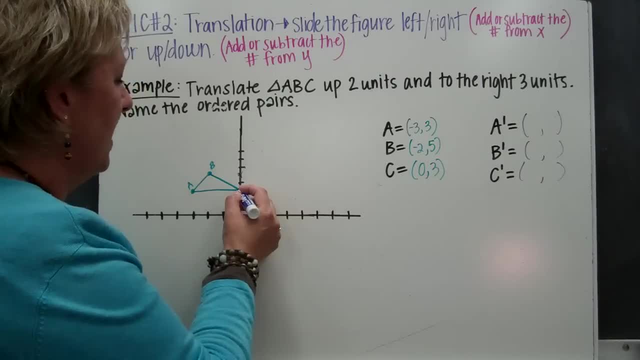 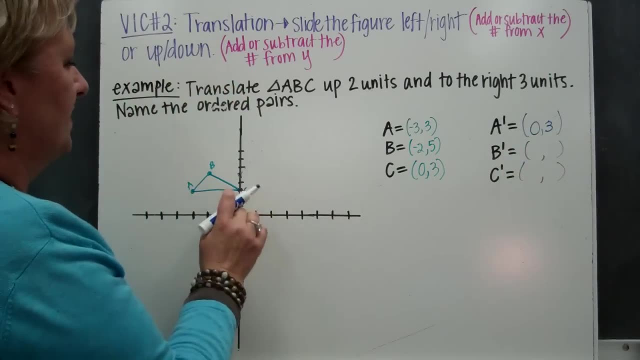 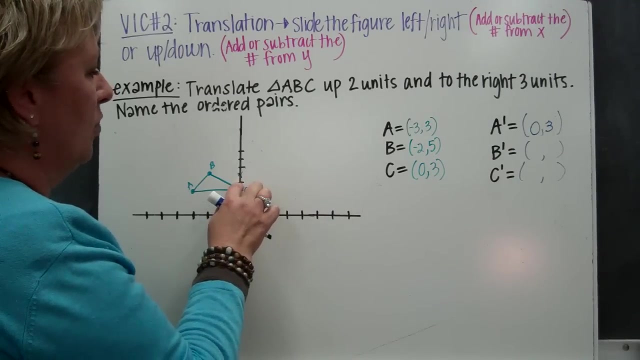 which will start it right here. okay, so I know that that is going to be 0, 3. okay, or? I'm sorry if I go over 3. I haven't even started doing it, right, I'm sorry. so if I go over 3 and up 2, it's going to go 1. 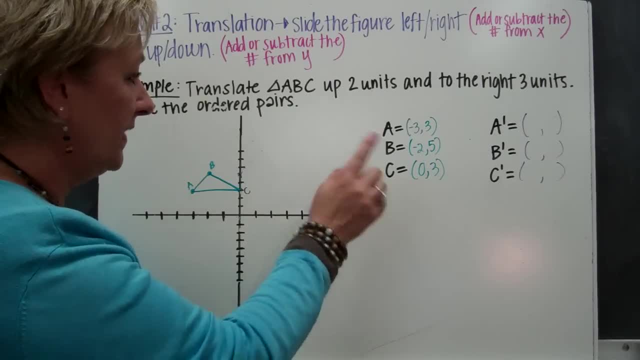 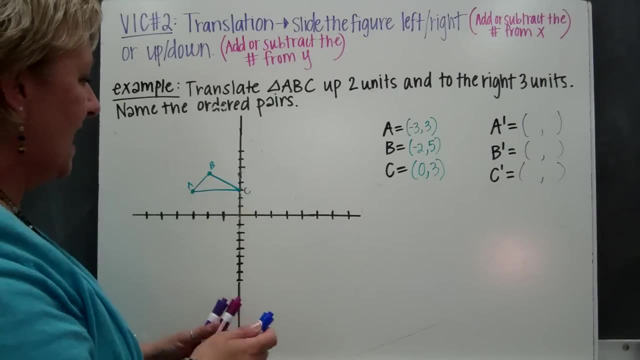 move it left to right on the X axis and three. If I want to change it by going up two and over to the right three, if I go take A and go to the right three, it's going to go over one, two, three on the Y axis, which will 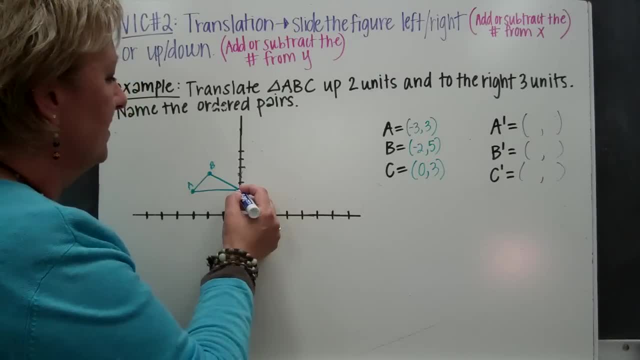 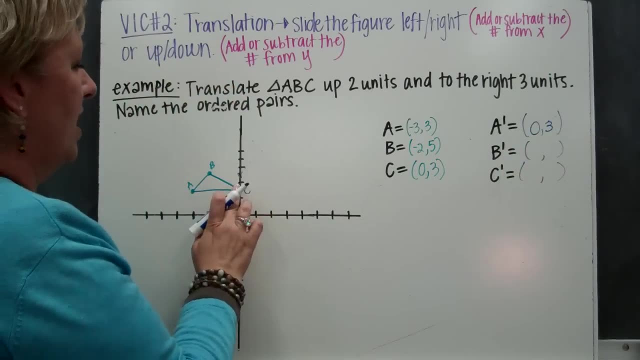 start it right here. I know that that is going to be zero three. I'm sorry if I go over three. I haven't even started doing it right. I'm sorry If I go over three and up two. it's going to go one over three and up two. the new A coordinate is going to be: 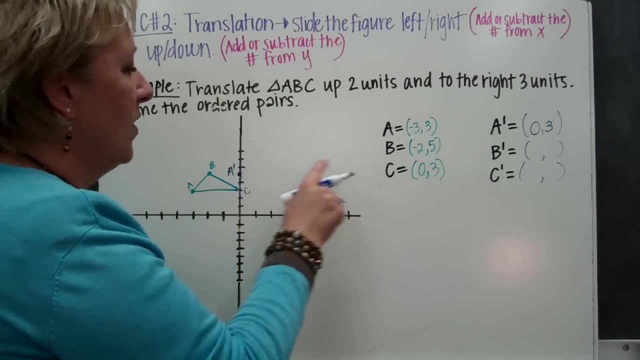 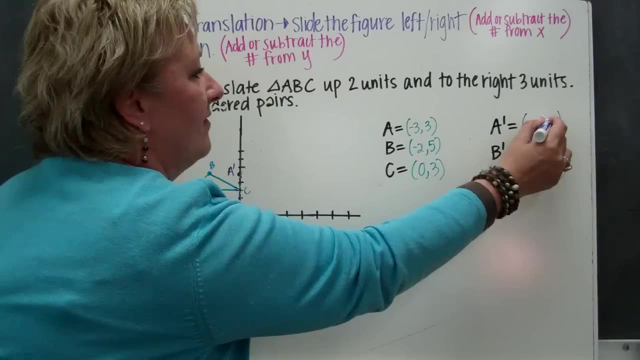 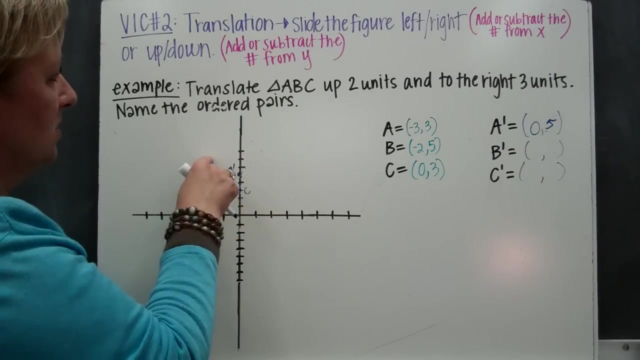 here. A prime is going to start here. I'm going to go over zero and one, two, three, four, five, Zero five. My new B is going to go up from here. It's going to go up one. 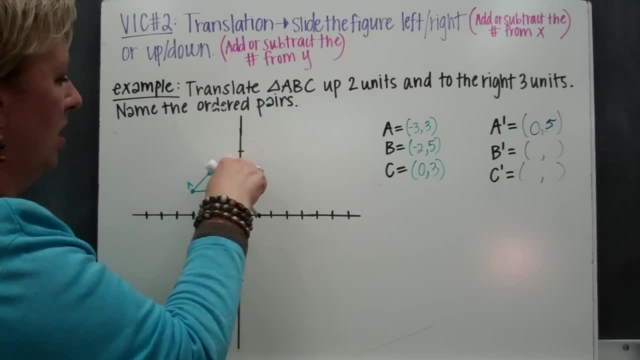 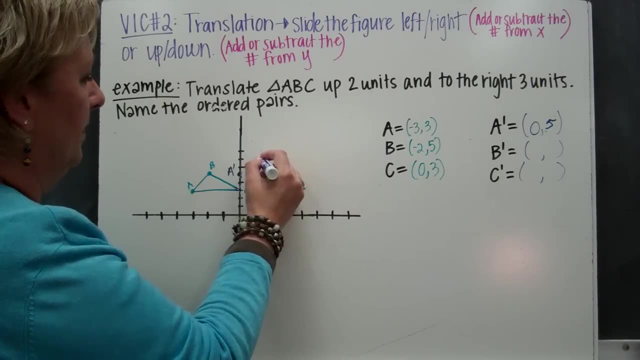 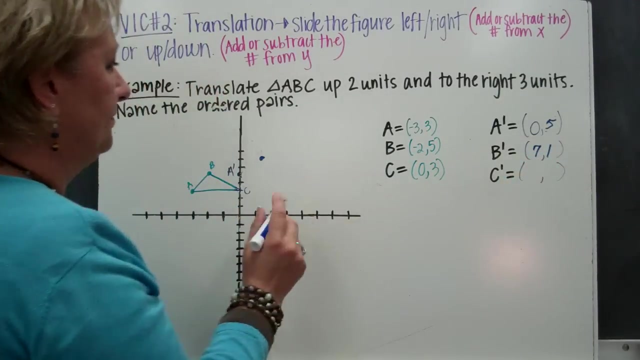 two and over to the right three, which is going to be one, two and three. This point is going to be over here at one, two, three, four, five, six, seven and one. I'm going to erase that so you can see that a little bit better. 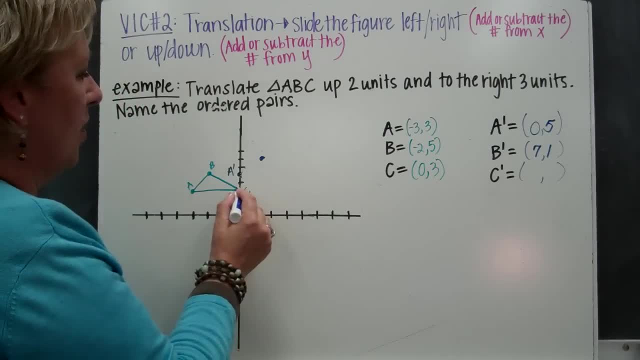 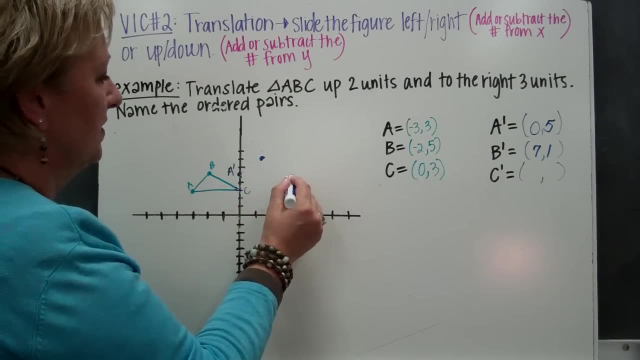 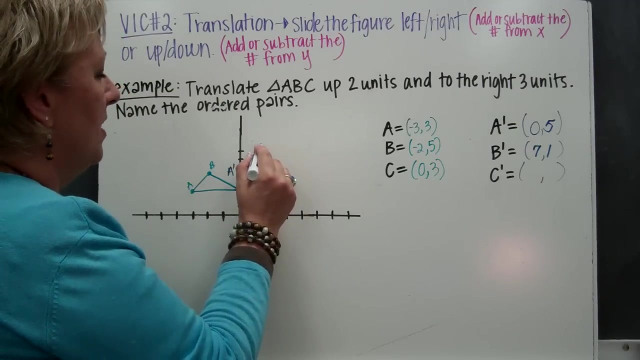 Then I'm going to put this over here. at C, It's going to go up one, two and over one, two, three units to the right. It's going to be right here. My new triangle is going to look like so this is a prime, B prime and C prime, and this is going to be one. 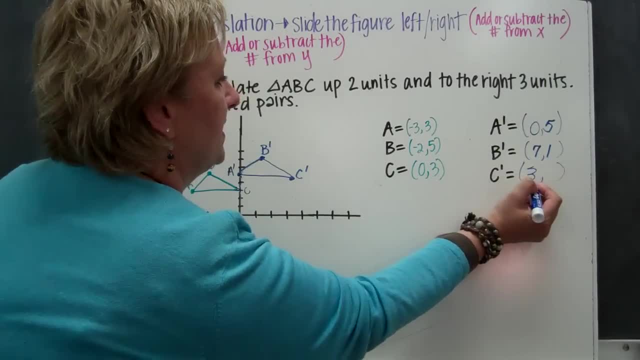 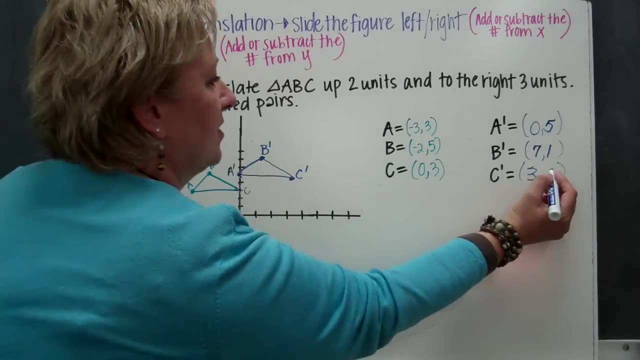 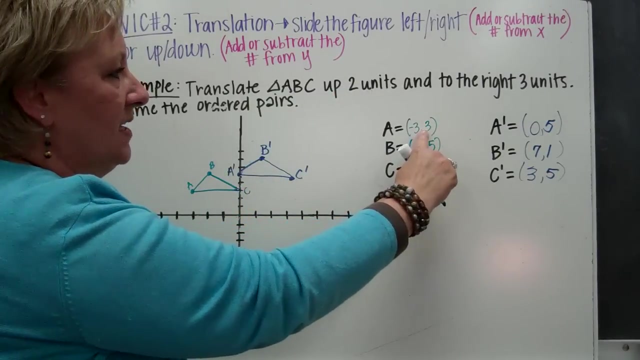 two, three over here for the C prime for this seat, for this three, and it's going to go up. one, two, three, four, five. so this is going to be three, five. if you notice, if I wanted to go up to, all I had to do was add two to each one of these and two. 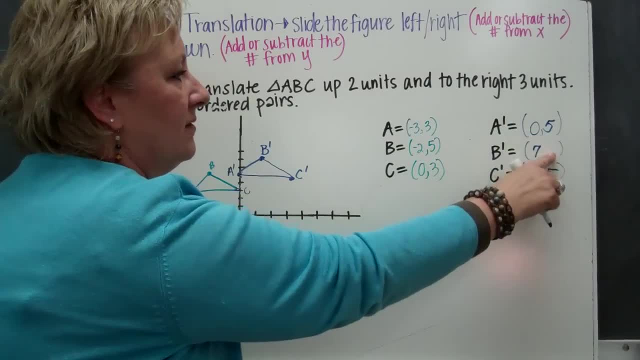 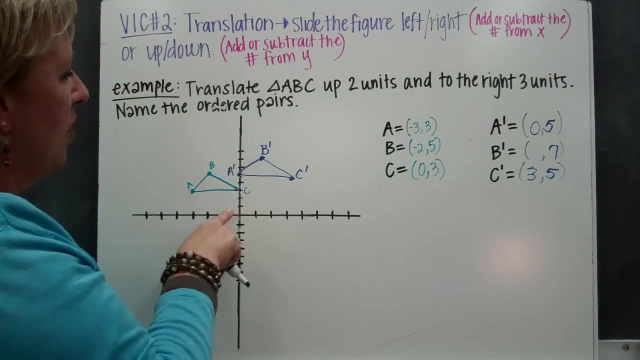 plus three is five. two plus five is seven. if I got that wrong, 2 plus five is seven and 2 plus three is five. if I wanted to go over to the right, if I wanted to go to the right three, I've got to move it three places with the X. so 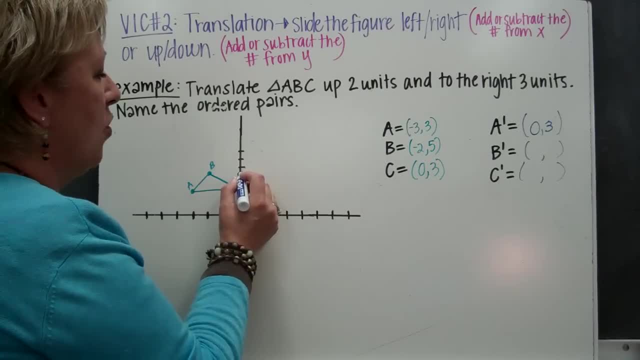 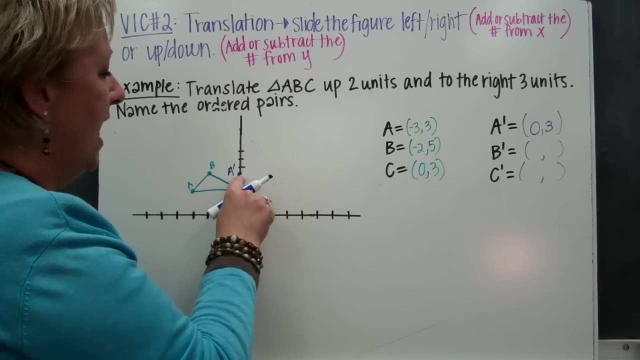 over 3 and up 2. the new A coordinate is going to be here, so A' is going to start here. so I'm going to go over 0 and 1, 2, 3, 4, 5, so 0, 5. 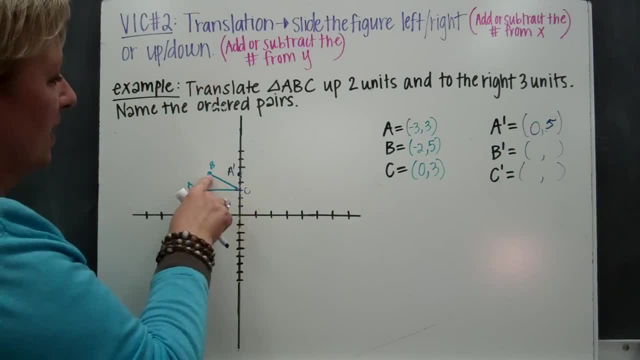 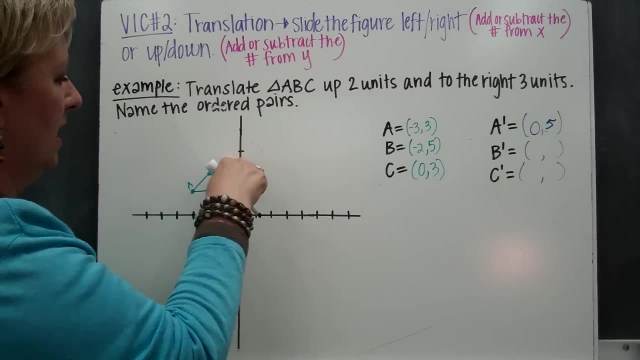 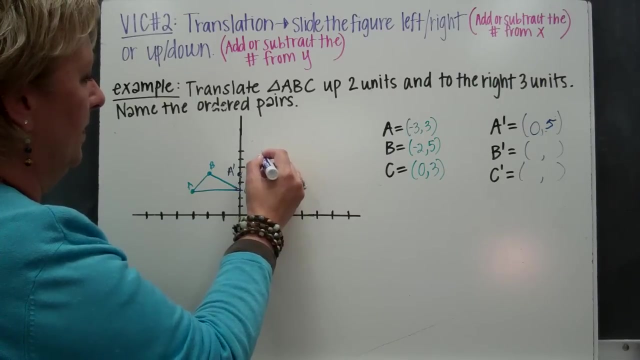 and my new B is going to go up from here. it's going to go up 1, 2 and over to the right 3, which is going to be 1, 2, 3. so this point is going to be over here at 1, 2, 3, 4, 5, 6, 7. 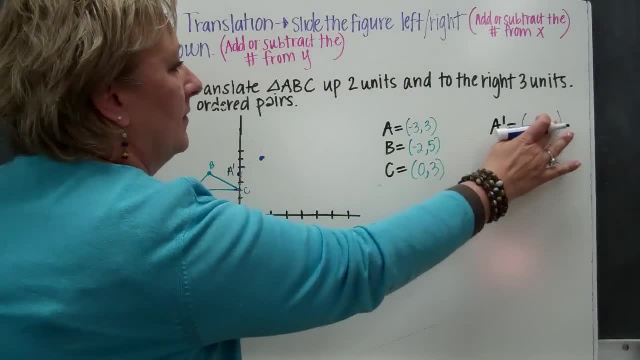 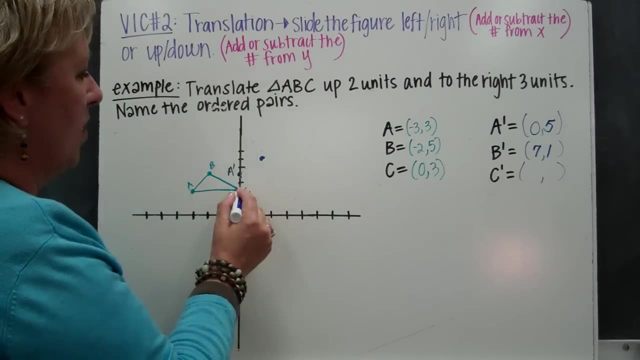 and 1. I'm going to erase that so you can see that a little bit better, and then I'm going to put this over here. at C it's going to go up 1, 2 and over 1, 2, 3 units to the right. 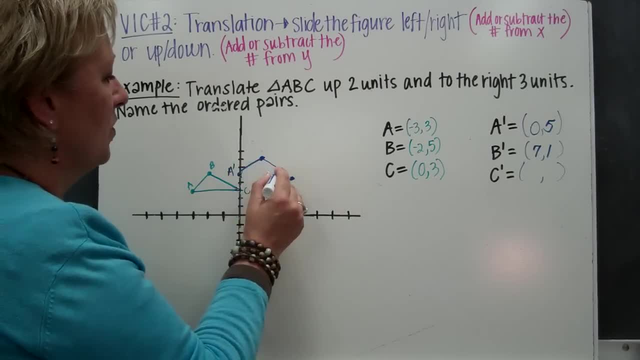 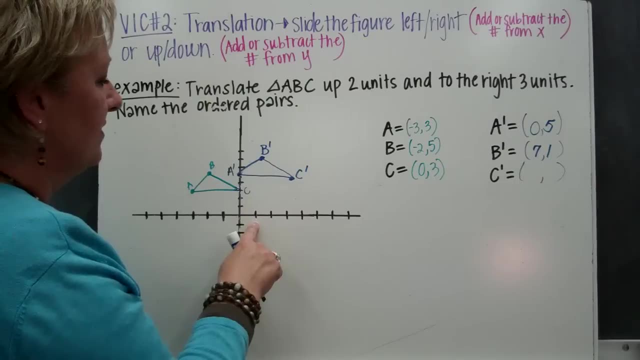 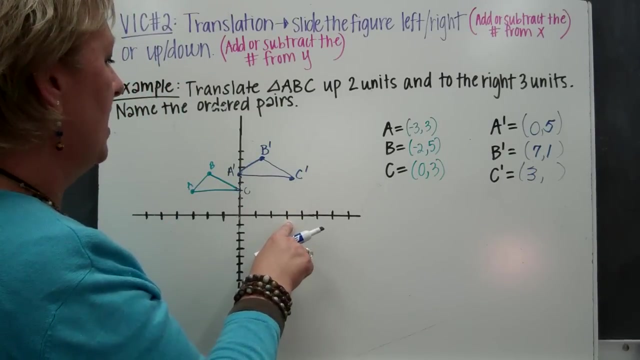 so it's going to be right here. so my new triangle is going to look like: so this is A', B' and C' and this is going to be 1, 2, 3 over here for the C', for this, for this 3, and it's going to go up. 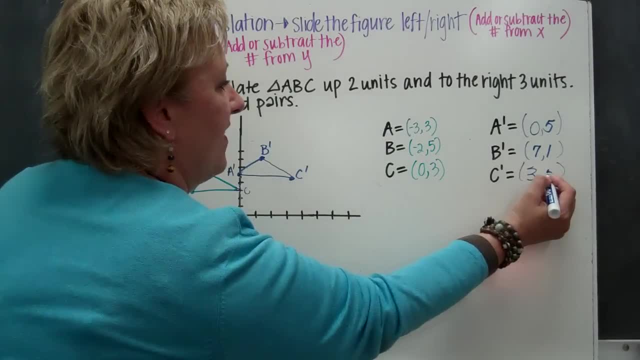 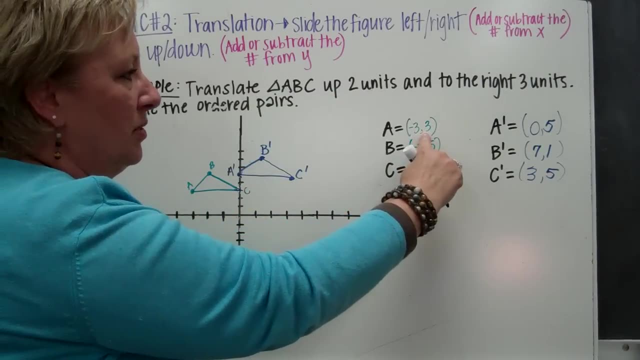 1, 2, 3, 4, 5, so this is going to be 3, 5, if you notice. if I wanted to go up 2, all I had to do was add 2 to each one of these, and 2 plus 3 is 5. 2 plus 3 is 5, so I'm going to add 2 to each one of these. 2 plus 3 is 5, so this is going to be 3, 5. 2 plus 3 is 5, so this is going to be 3, 5. 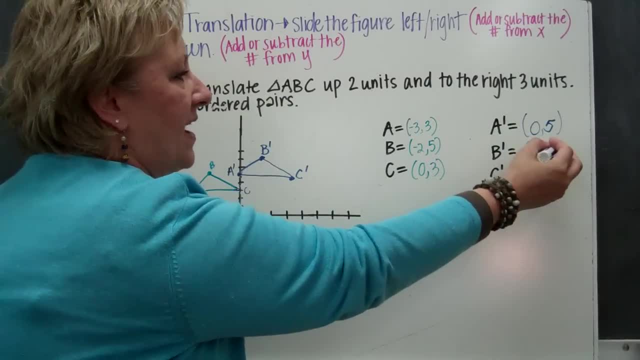 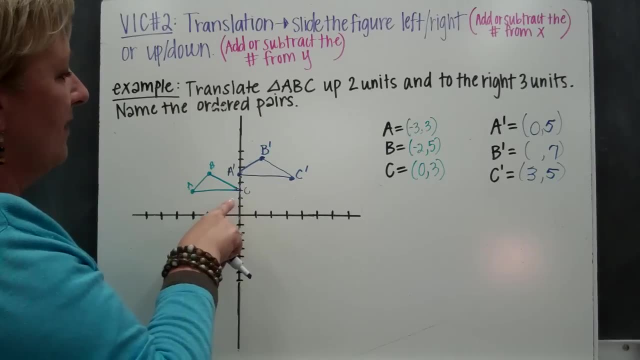 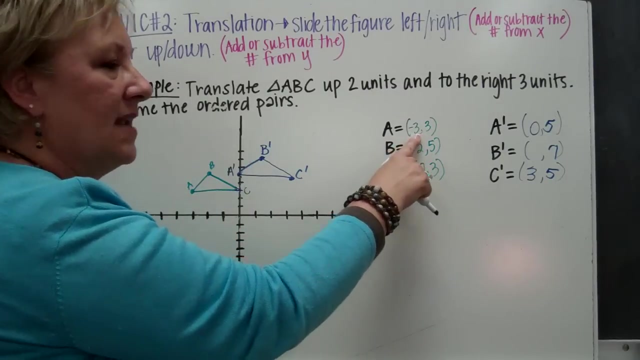 so this is going to be 3, 5, 5 is 7, and 2 plus 3 is 5.. If I wanted to go over to the right 3, I've got to move it 3 places with the x. so with the a I'm going to add 3, so that negative 3 plus 3 gives. 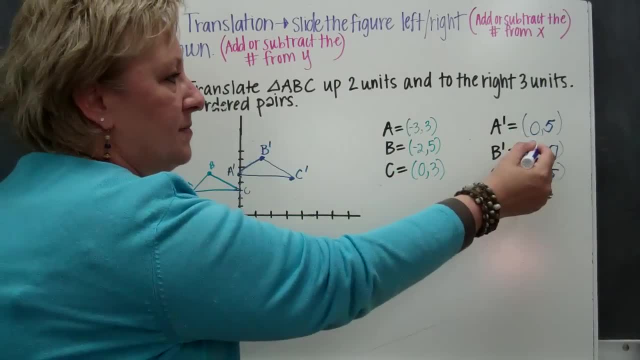 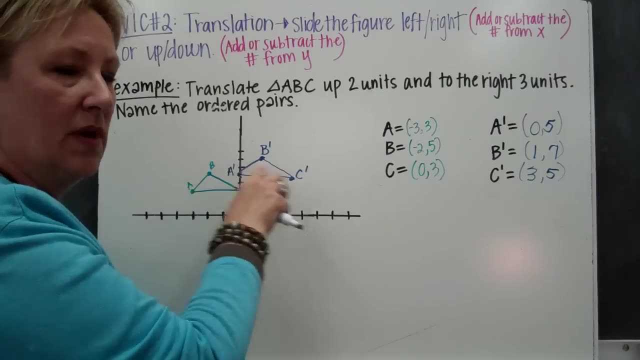 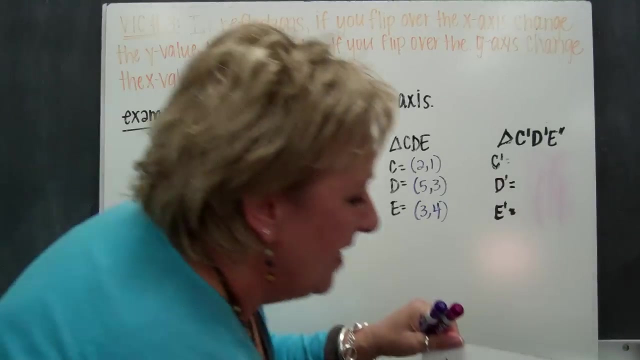 me 0, negative 2 plus 3 gives me 1, and 0 plus 3 gives me 3.. So I can either add it to my coordinates or I can do it on the graph. as such Very important concept number 3.. In a reflection, if you flip over the x-axis, you're going. 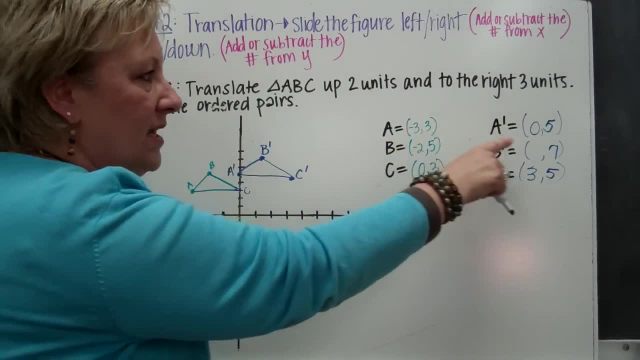 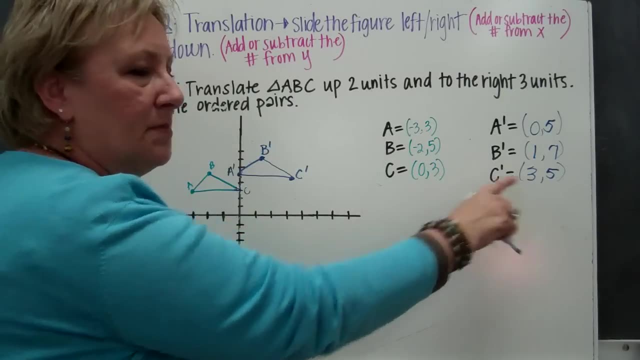 with the a I'm going to add three, so that negative 3 plus 3 gives me 0, negative 2 plus 3 gives me 1, and 0 plus 3 gives me 3. so I can either add it to my course or vice versa, so I can become the maximum prime. so if Iתח, so I can. 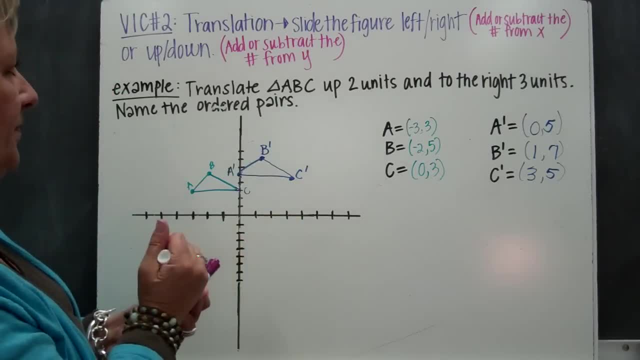 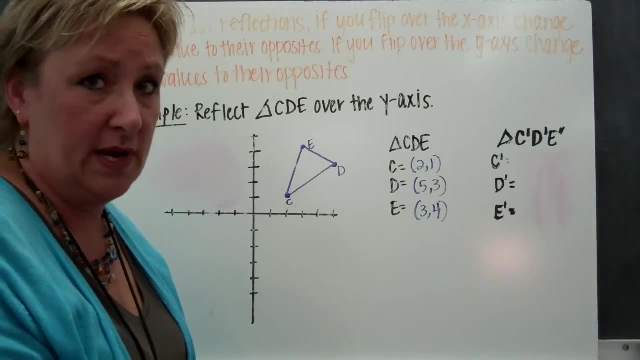 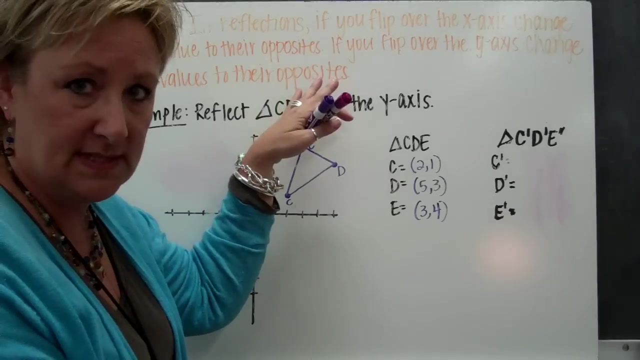 either add it to my course or vice versa. so I sigma plus nine, it would be one coordinates where I can do it on the graph as such Very important concept. number three: In a reflection, if you flip over the x-axis, you're going to change the y-value to their opposites, And if you flip over the y-axis, you're going 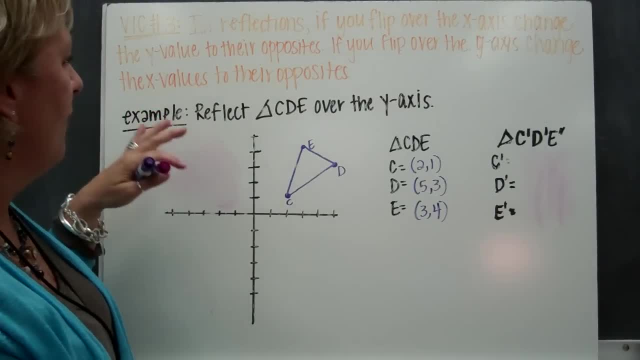 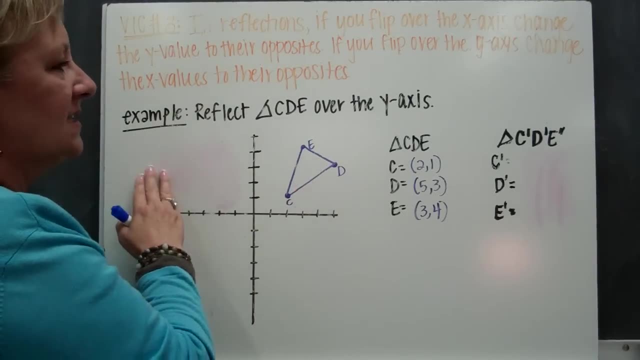 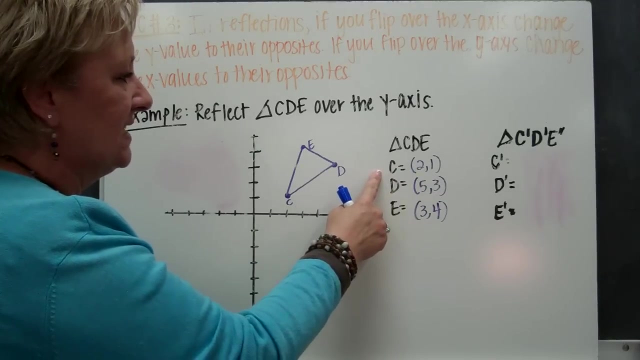 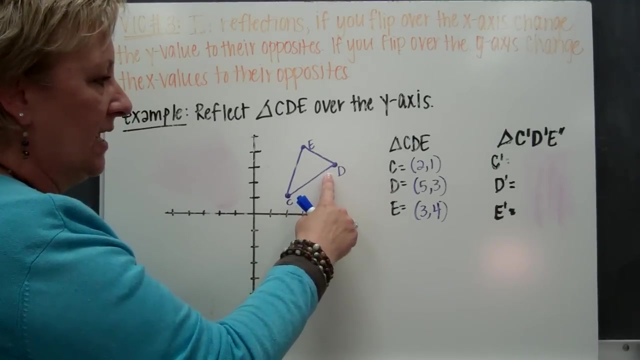 to change the x-values to their opposites. For example, let's look at the triangle C-D-E and we're going to reflect it over the y-axis here. So I've got triangle C-D, angle C is going to be at 2 and 1,, triangle D is going to be at 5 and 3, and angle E is going to. 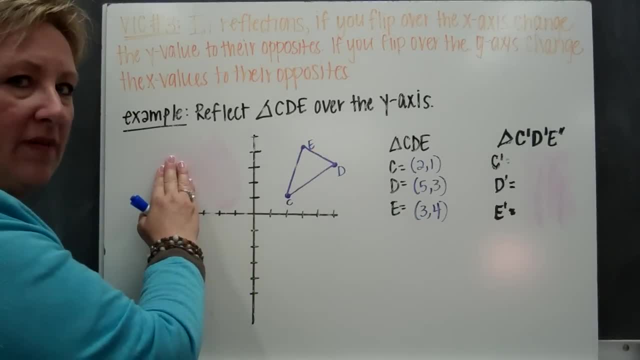 be at 3 and 4.. And if I'm going to flip it or reflect it over the x-axis, I'm going to change the x-value to their opposites, it over this y-axis here. that's the up and down. then what I've got to do is, when I turn 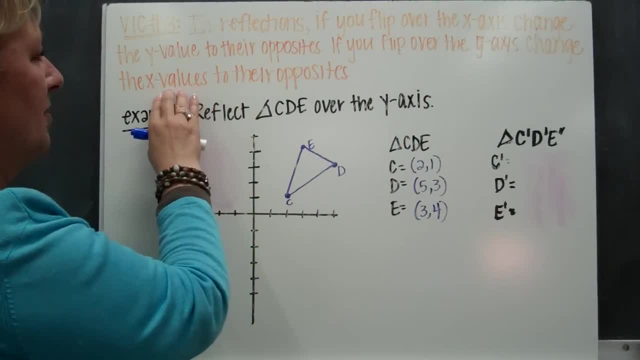 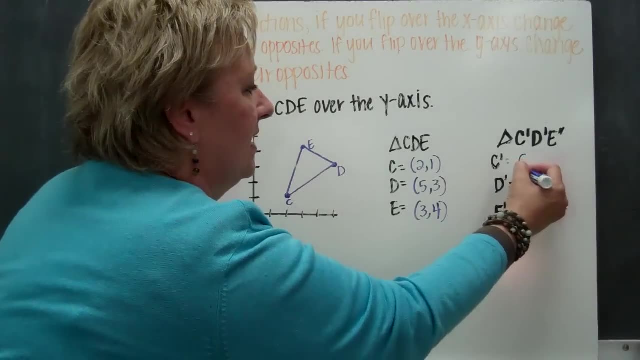 it over. when I flip it over the y-axis I'm going to make, the x's are going to be their opposites. So if x is 2 here, I know that in this case it's got to be negative 2 and. 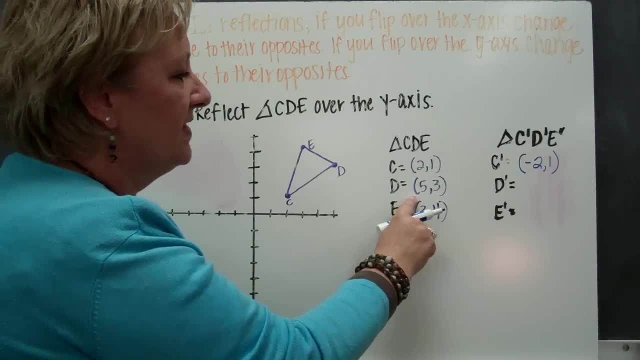 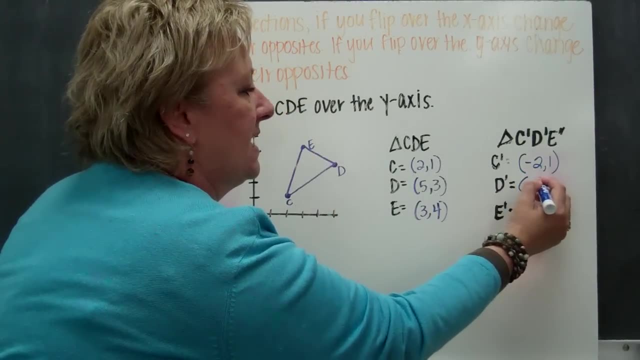 1. I'm going to keep the y's the same. If d is 5, the original image is 5, then I know that its prime image is going to be at negative 5 and 3.. And I know, if e is at 3,, its prime 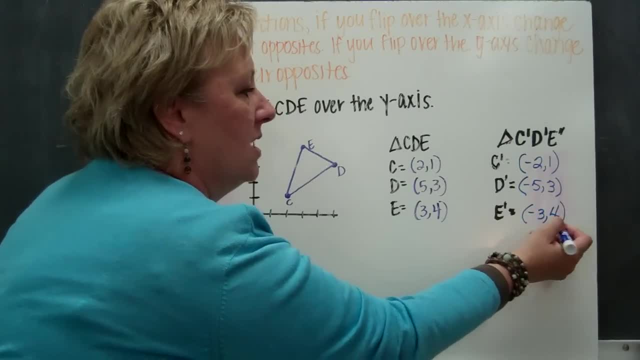 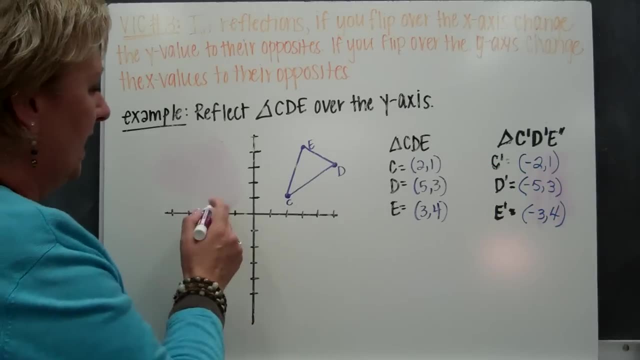 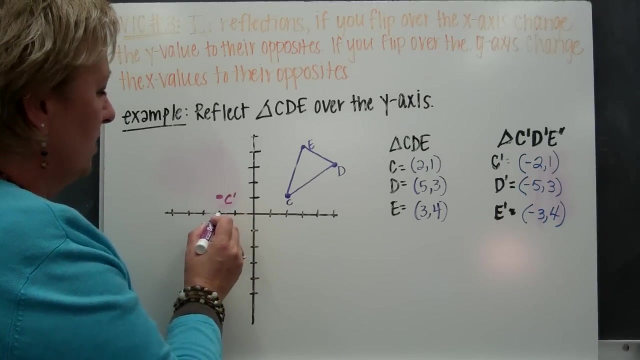 image is going to be at negative 3 and 4.. So when I go to graph these it's going to look like a negative 2 and 1.. Negative 2 and 1 is my new prime c. Negative 5, 1,, 2, 3,. 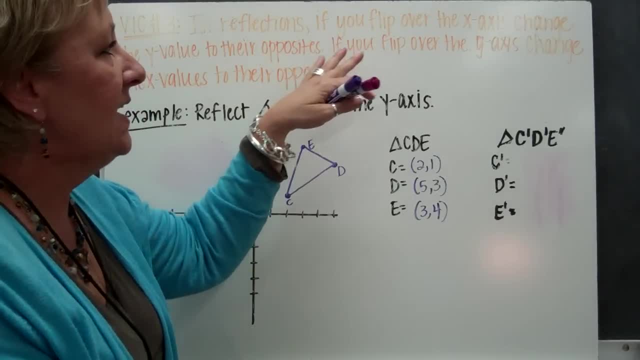 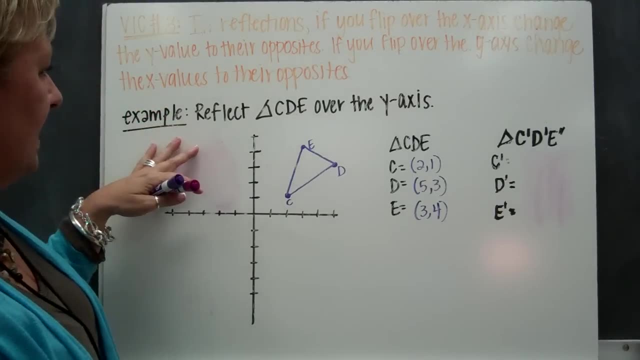 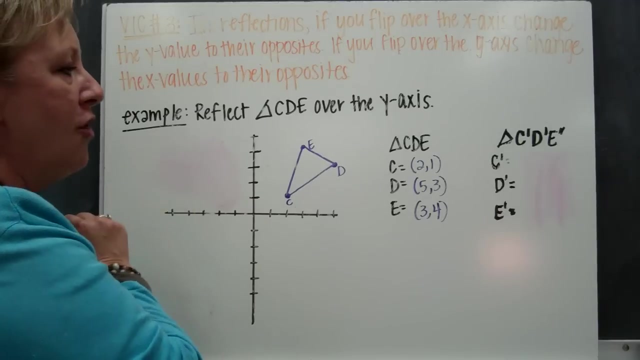 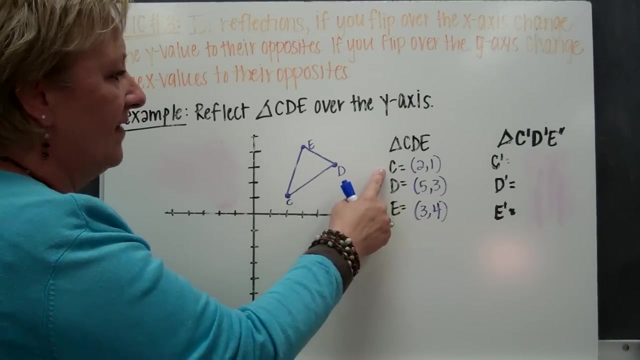 to change the y-value to their opposites. and if you flip over the y-axis you're going to change the x-values to their opposites. For example, let's look at the triangle C and Y. We're going to reflect it over the y-axis here. So I've got triangle CD. angle C is 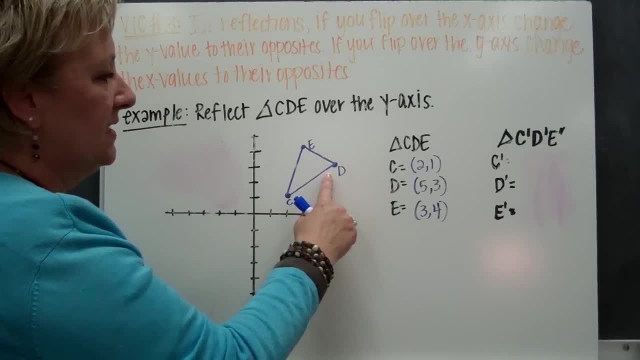 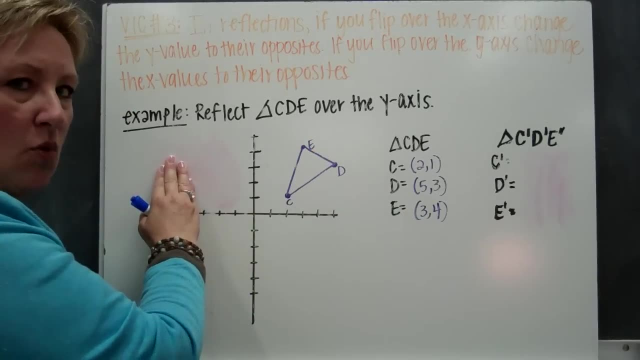 going to be at 2 and 1,, triangle D is going to be at 5 and 3, and angle E is going to be at 3 and 4.. And if I'm going to flip it or reflect it over this y-axis here, that's: 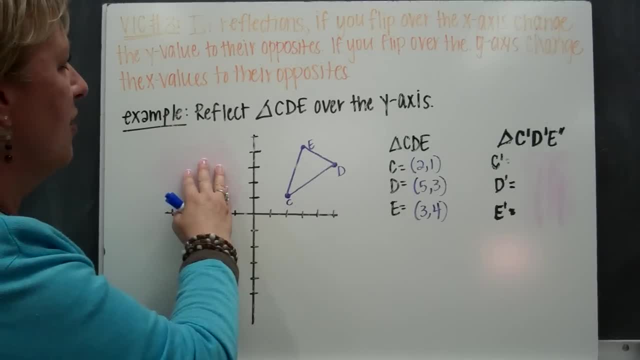 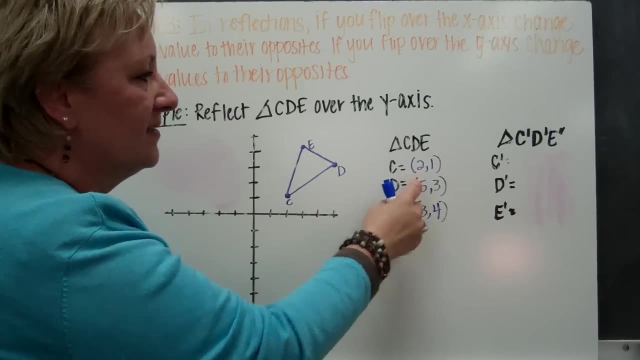 the up and down, then what I've got to do is, when I turn it over, when I turn it over, when I flip it over, the y-axis I'm going to make the x's are going to be their opposites. So if x is 2 here, I know that in this case it's got to be negative 2 and 1. I'm going. 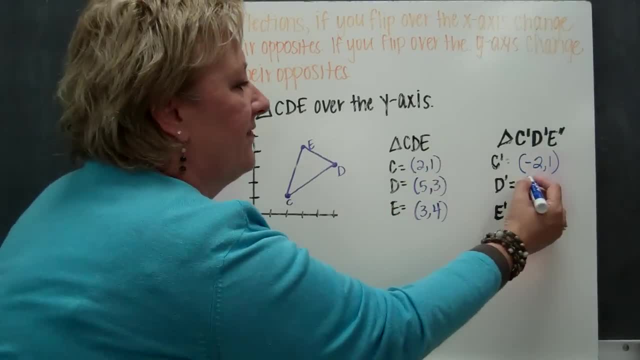 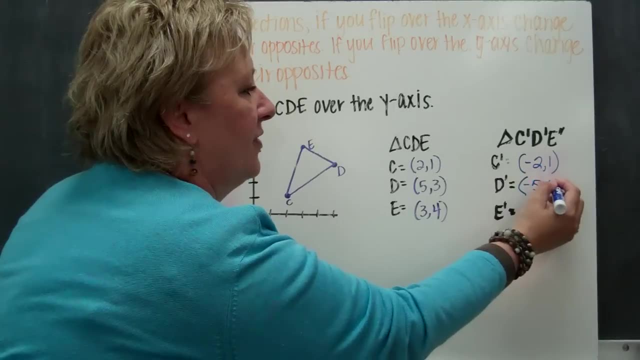 to keep the y's the same. If D is 5,, the original image is 5, then I know that its prime image is going to be at negative 5 and 3.. And I know if E is at 3, its prime image is going. 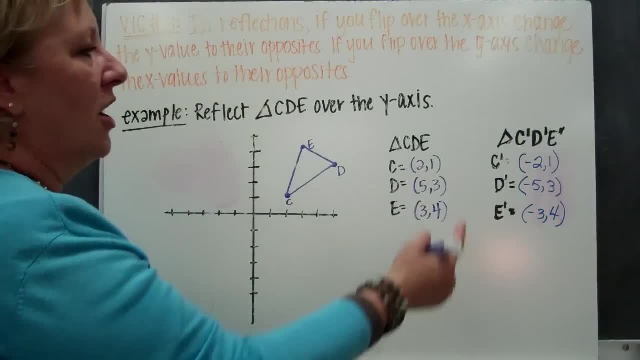 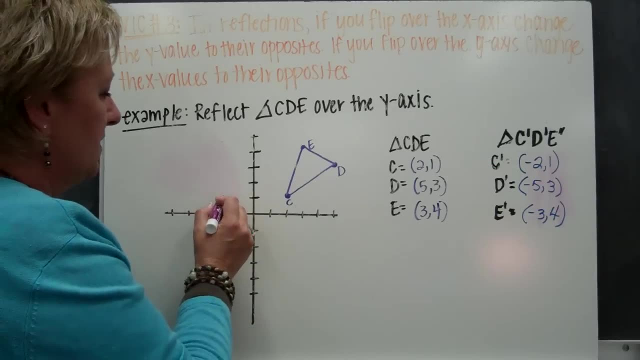 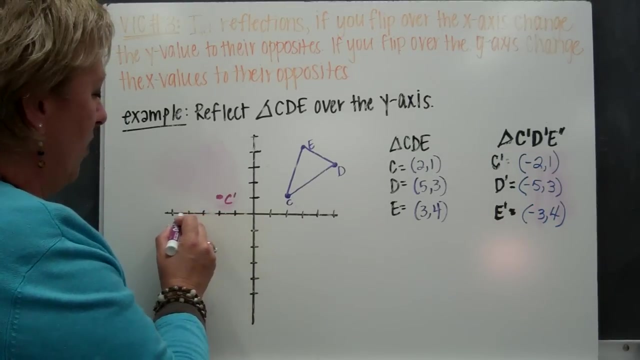 to be at negative 3.. So when I go to graph these, it's going to look like a negative 2 and 1.. Negative 2 and 1 is my new prime. C. Negative 5, 1, 2,, 3,, 4, 5, and 3, 1,, 2, 3, is going to be my new prime. 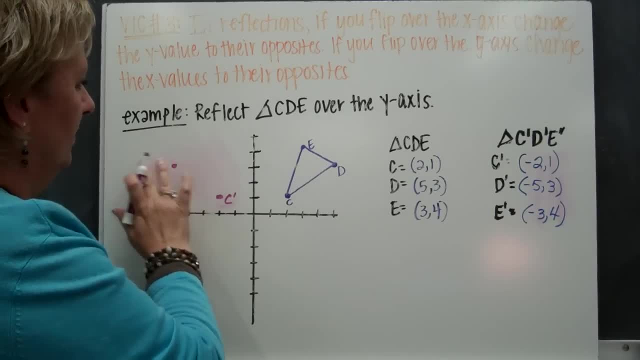 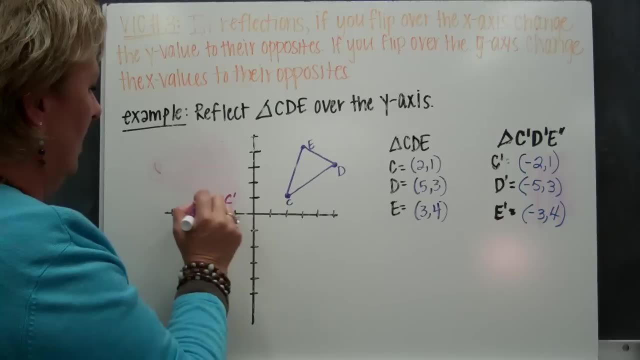 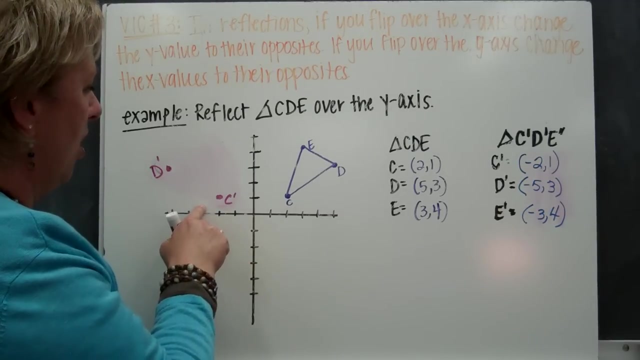 E, D And this is going to be my new prime D And I know that negative 3, 1,, 2,, 3, and 4, 1,, 2,, 3,, 4, is going to be my new prime E. 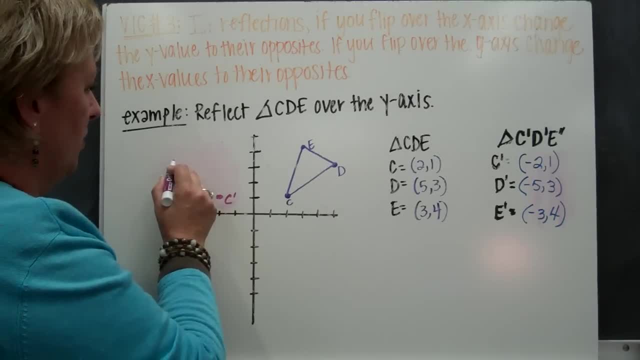 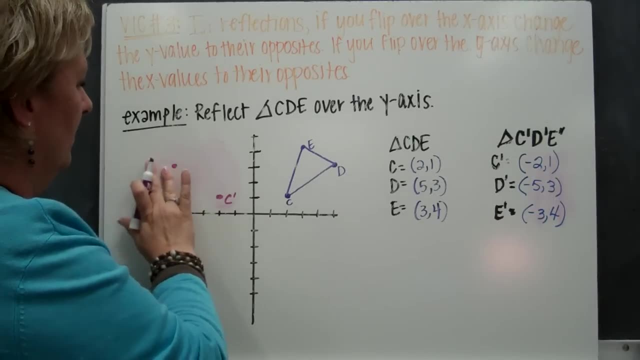 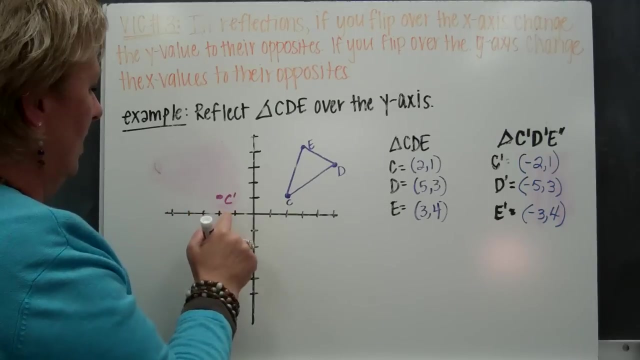 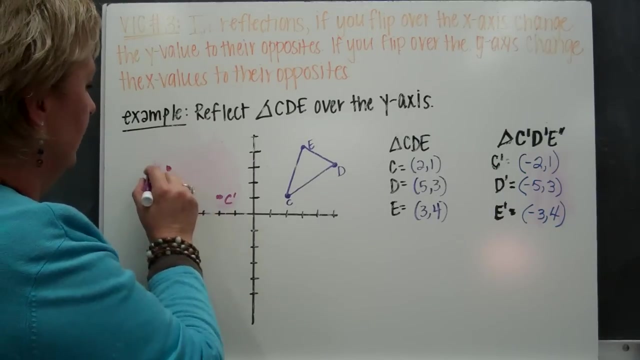 4,, 5, and 3,. 1,, 2,, 3, is: 1. going to be my new prime E D: 1,, 2,, 3,, 4,, 5, and 3.. 1,, 2,, 3.. And this is going to be. 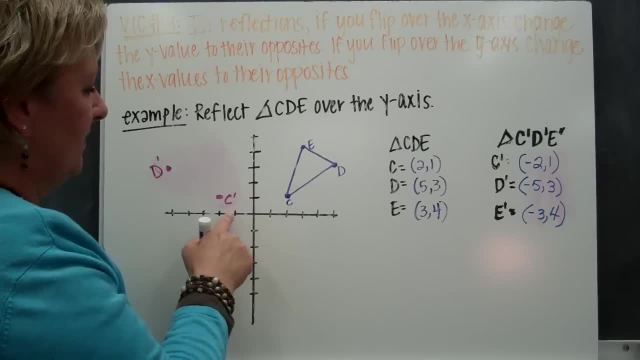 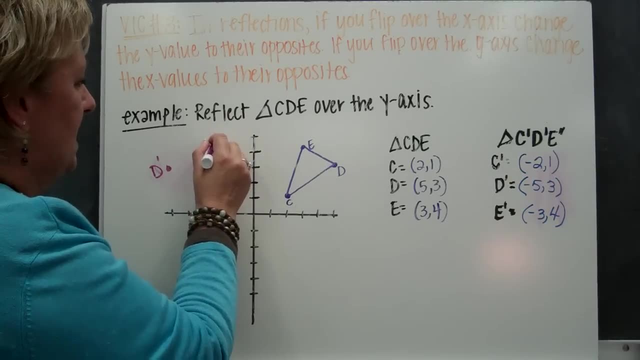 my new prime D And I know that negative 3, 1,, 2,, 3, and 4, 1,, 2,, 3, 4, is going to be my new prime E And I'm going to connect these together and these are going to just be a. 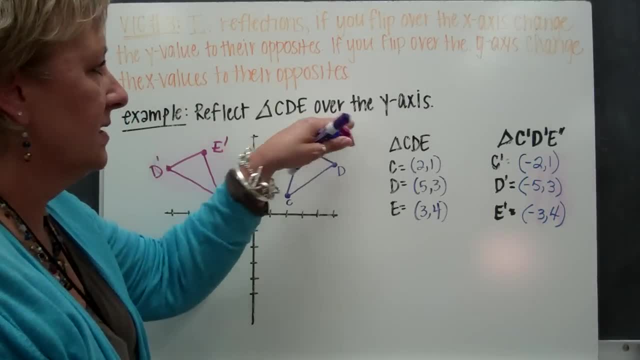 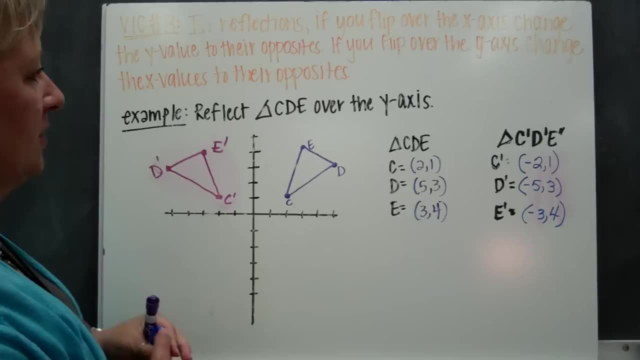 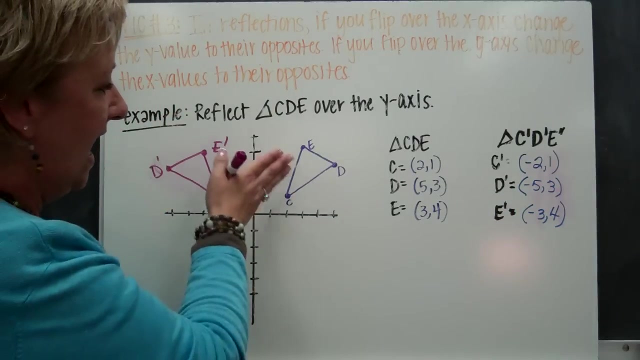 flip-flop over the y-axis of what we started out here with my first image and my prime image. So we're only going to do it. if I flipped over the y-axis, It was only going to change my x-axis to the opposite. Had I flipped over the x-axis, my y's would have turned into. 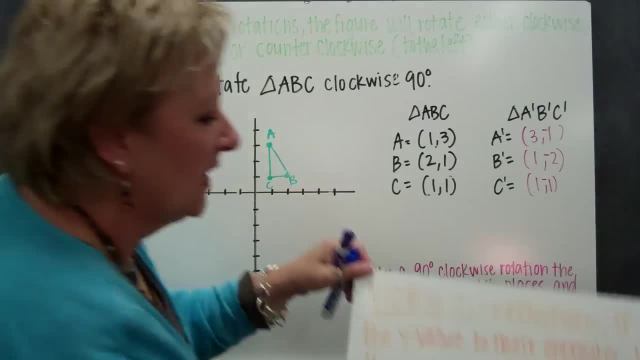 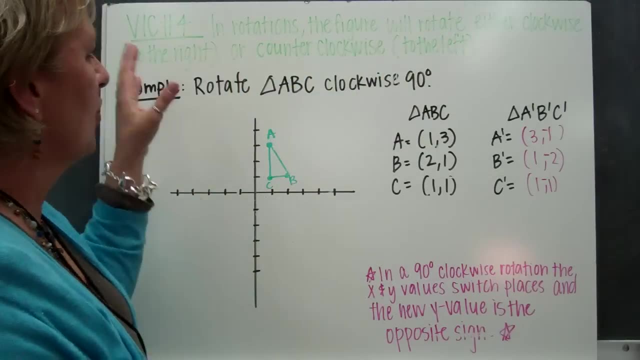 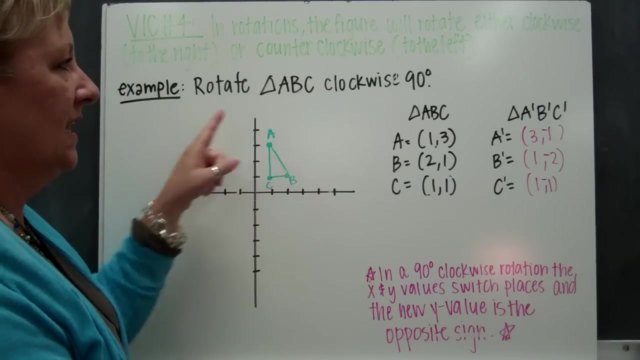 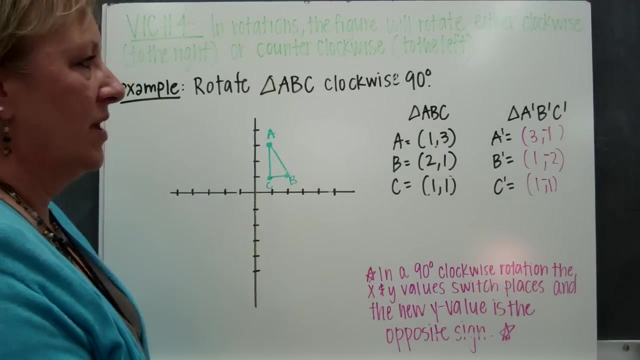 the negative, Very important concept. number four: In rotations, the figure will rotate either clockwise meaning to the right or counterclockwise meaning to the left. In this case we're going to rotate triangle A, B, C into a 90-degree angle. So when I'm doing this, I'm going to look. 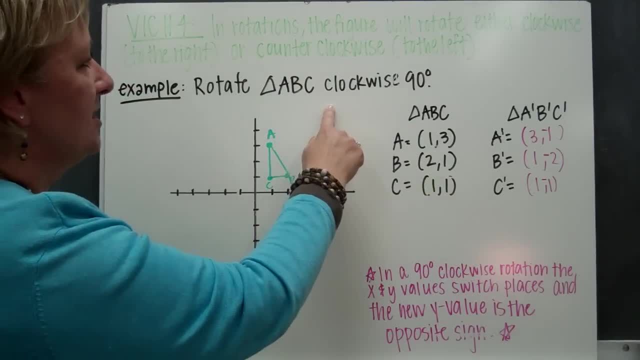 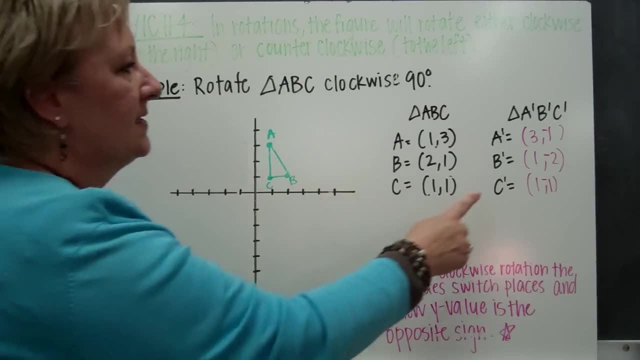 at angle 1.. And this is going to change because this is now going to be flipped and the A is going to be over here. So if I'm looking at this, I'm going to flip my x value with my y value. 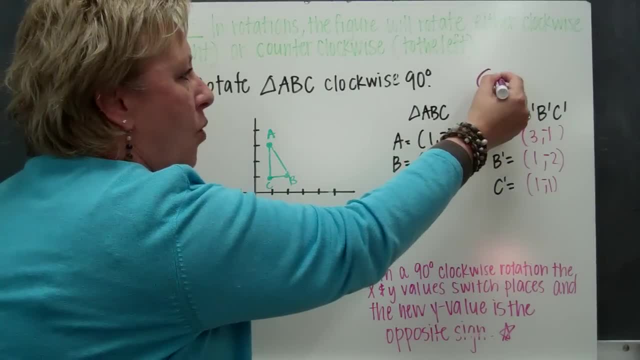 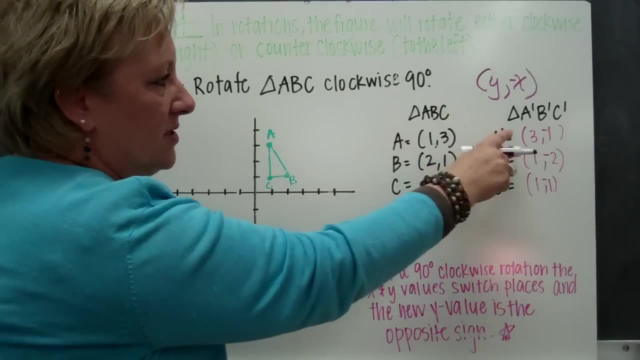 So instead of 1,, 3,, it's now going to look like y, x and the x value is going to be negative. That's all we did from here to here. So from 1,, 3,, it's going to be 3, negative. 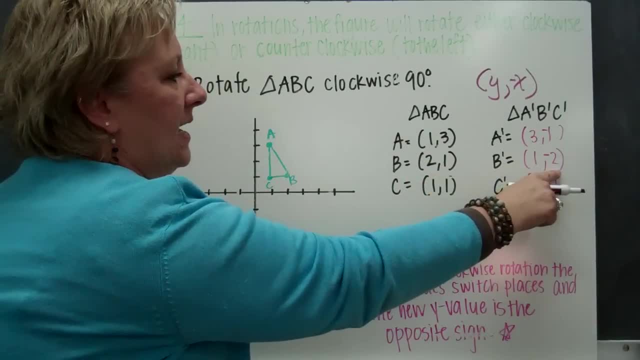 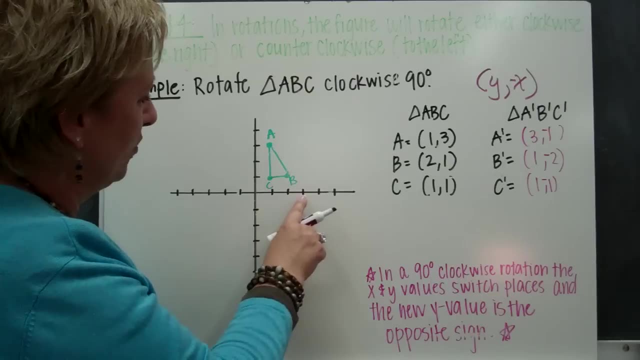 1.. For 2, 1, it's going to be 1, negative 2.. And for 1, 1, it's just going to be 1, negative 1.. So when I go to graph the prime of these, it's going to be 3, negative 1.. It's going. 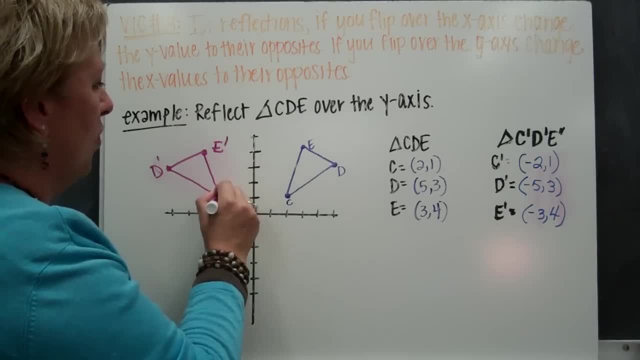 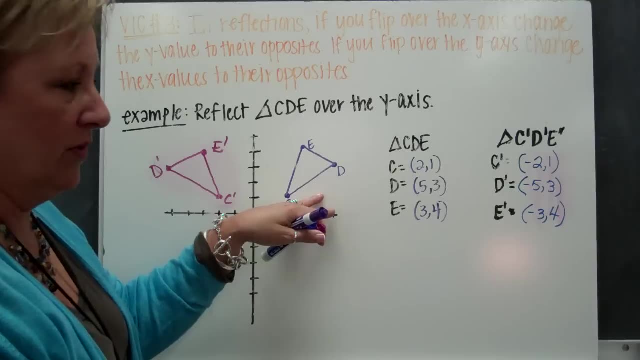 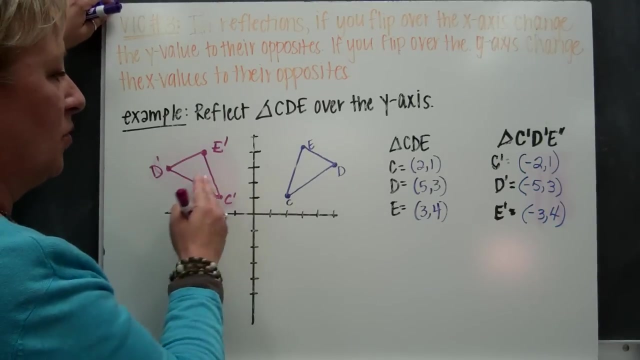 And I'm going to connect these together and these are going to just be a flip-flop over the y-axis of what we started out here with my first image and my prime image. So we're only going to do it if I flipped over the y-axis. 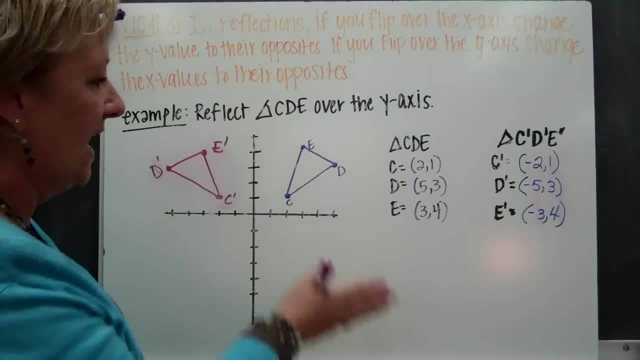 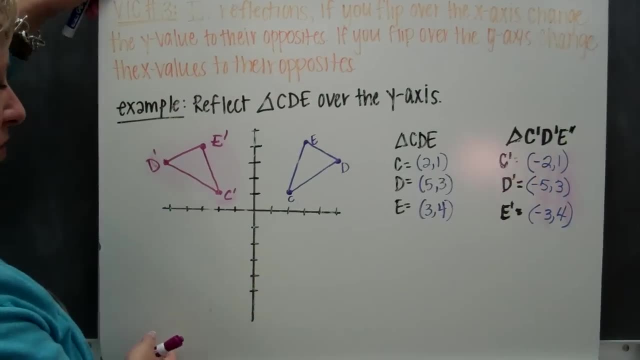 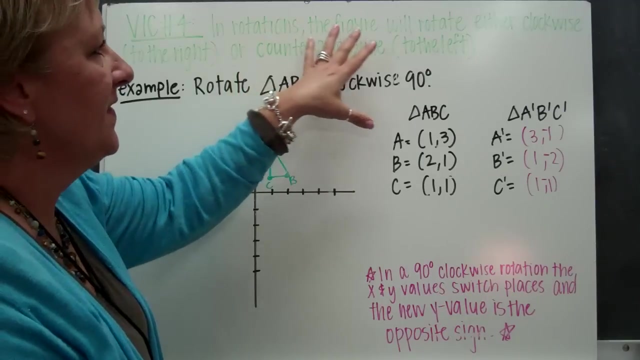 It was only going to change my x-axis to the opposite. Had I flipped over the x-axis, my y's would have turned into the negatives of what we started with. Very important concept number four: In rotations, the figure will rotate either clockwise meaning to the right. 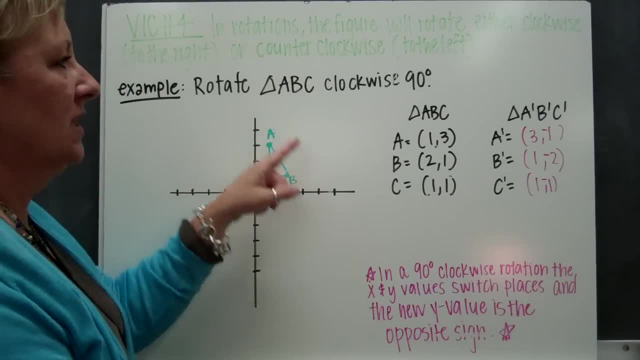 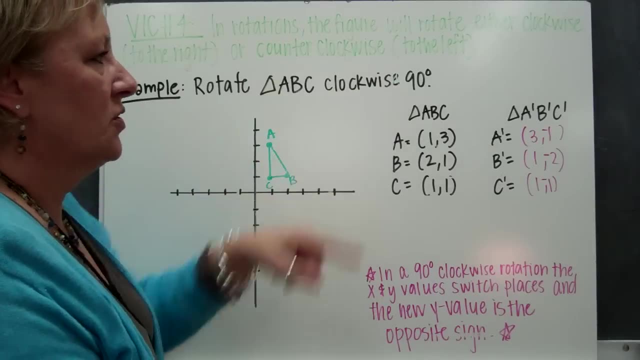 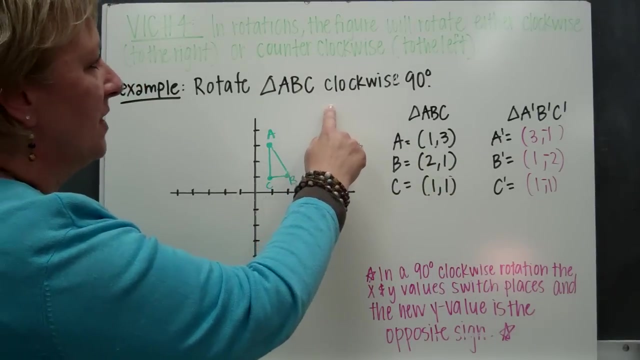 or counterclockwise meaning, to the left In this case, we're going to rotate triangle ABC into a 90-degree angle. So when I'm doing this, I'm going to look at angle one. This is going to change because this is now going to be flipped. 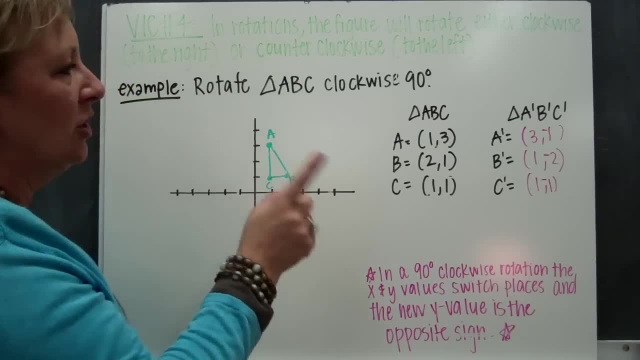 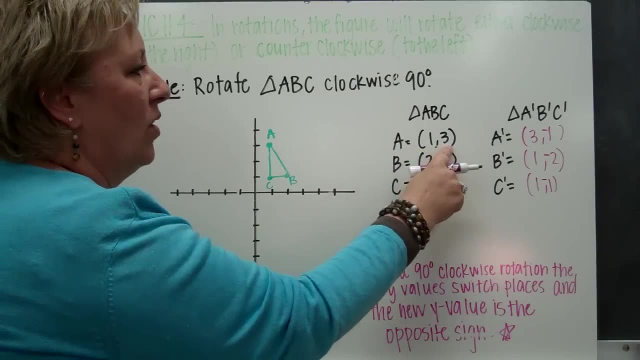 and the A is going to be over here. So if I'm looking at this, I'm going to flip my x value with my y value. So instead of 1,, 3, it's now going to look like y, x. 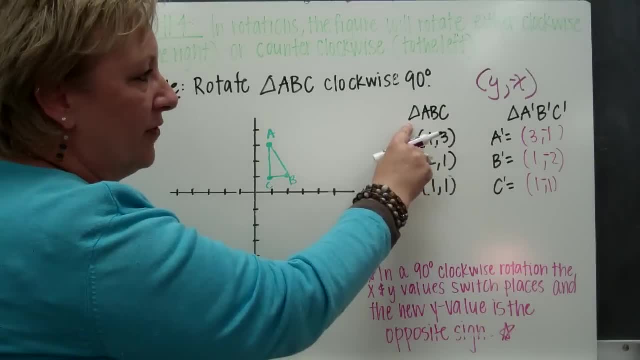 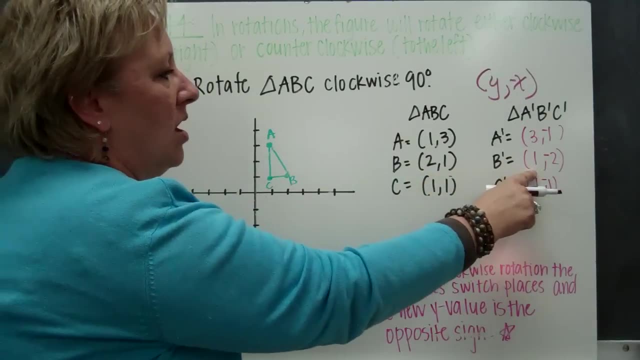 and the x value is going to be negative. That's all we did from here to here. So for 1,, 3,, it's going to be 3, negative 1.. For 2, 1, it's going to be 1, negative 2.. 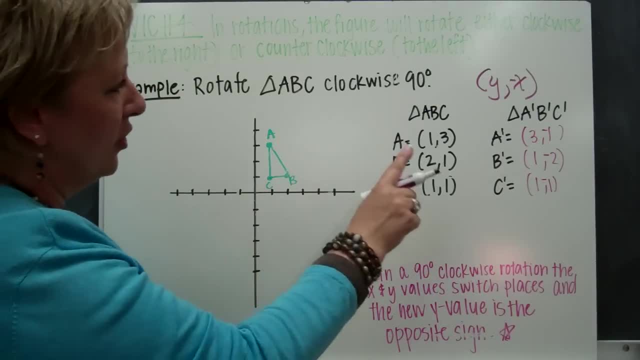 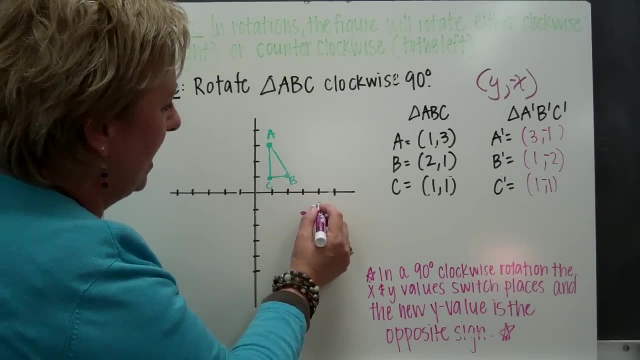 And for 1, 1, it's just going to be 1, negative 1.. So when I go to graph, the prime of these is going to be 3, negative 1.. It's going to be my A prime. 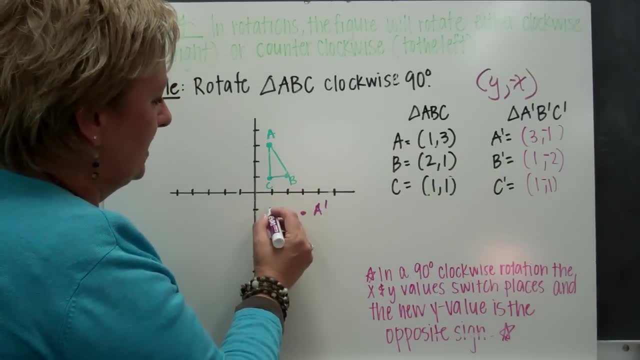 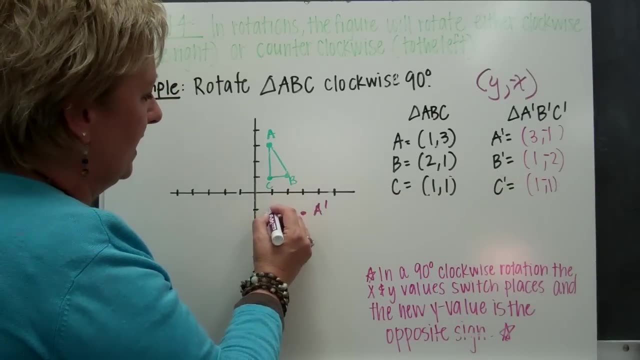 B, my prime B is going to be 1, negative 2, which is my B value here prime, And C is going to be 1, negative 1, which is my C prime, And I'm going to connect these together. 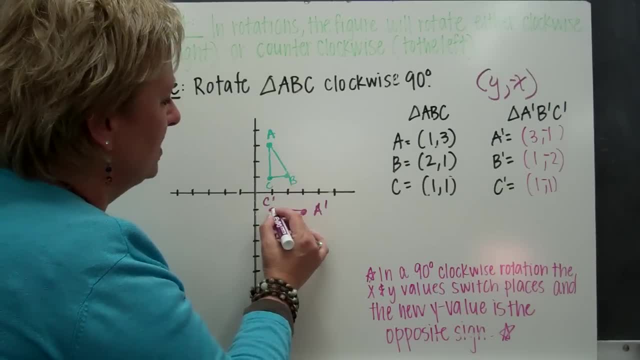 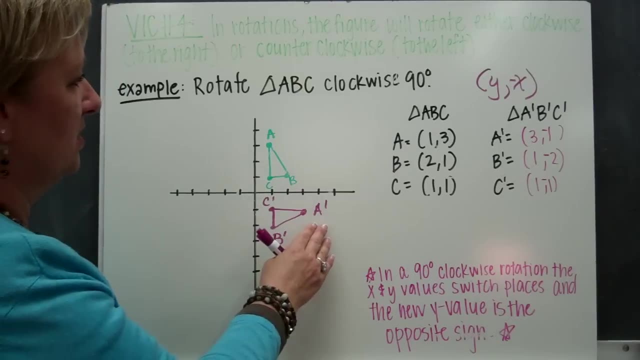 And when I do, I have rotated this in a 90-degree angle down into the triangle And I'm going to connect this in a 90-degree angle down into quadrant 4, which is going to be- I mean, yes, 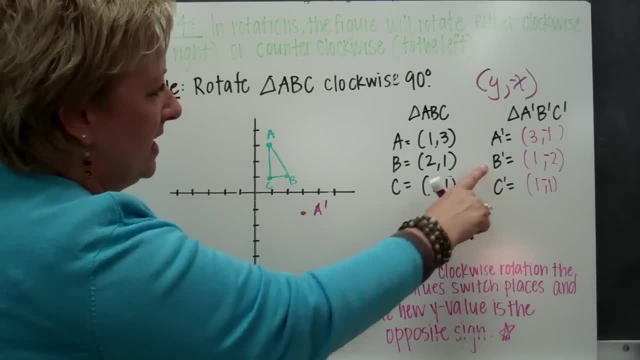 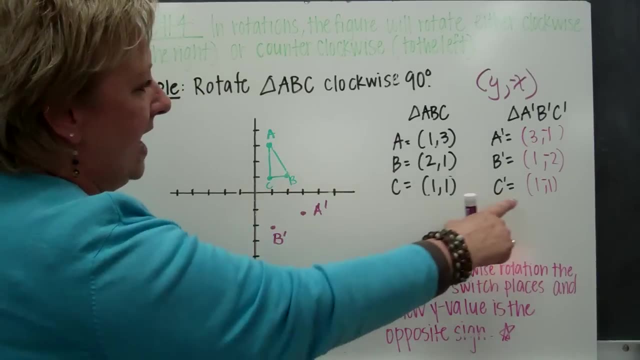 to be my A prime. My prime B is going to be 1, negative 2,, which is my B value here prime, And C is going to be 1, negative 1,, which is my C prime, And I'm going to connect these. 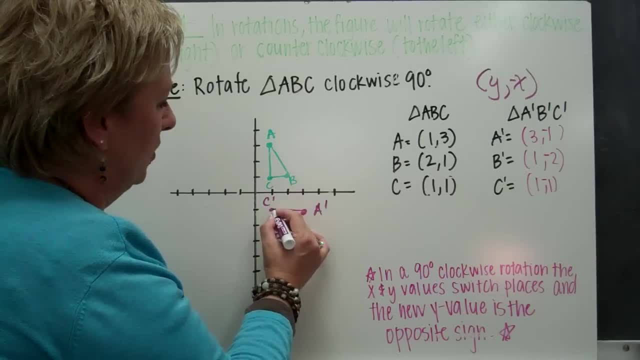 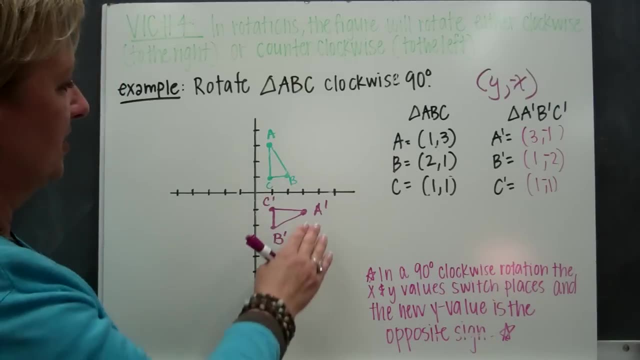 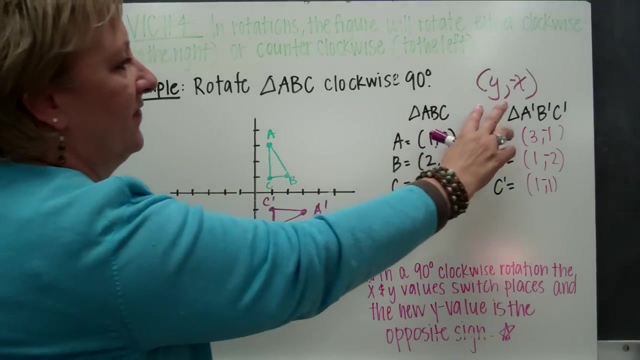 together. And when I do, I have rotated this in a 90 degree angle down into quadrant 4,, which is going to be- I mean yes- which is going to be- quadrant 2, which is going to be positive, negative Because I have flipped my 2 x's and y's over and I have made my 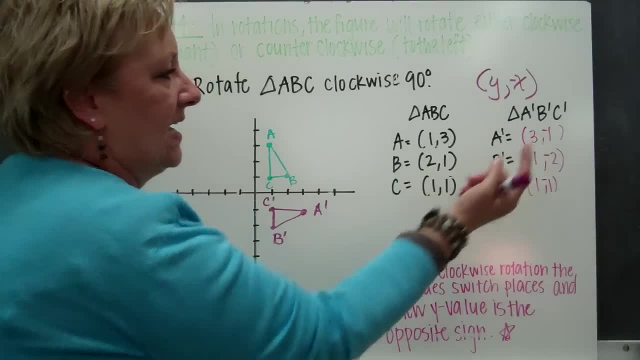 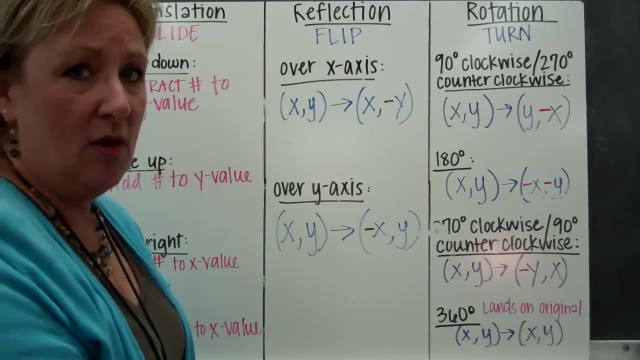 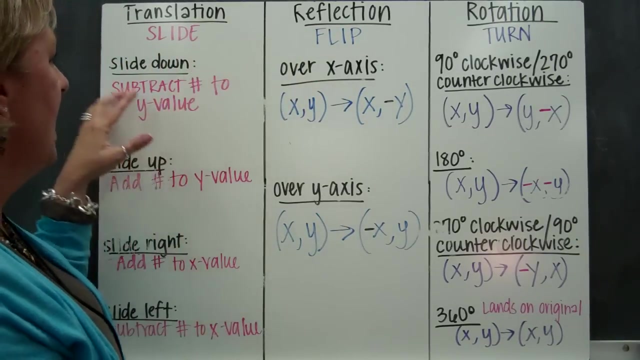 x value, which is now in the y's position, a negative. This is just to recap what we've talked about. When we're talking about translations, we're talking about sliding the image either left or right or up and down. When I am sliding, 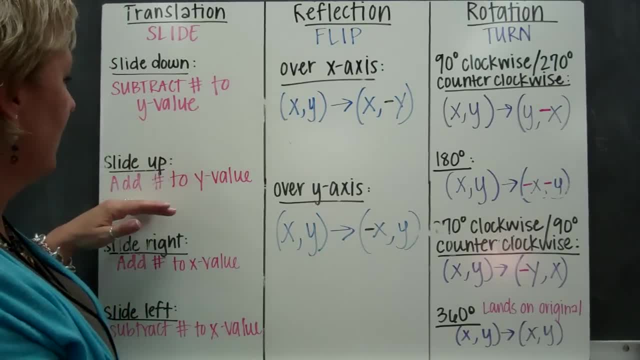 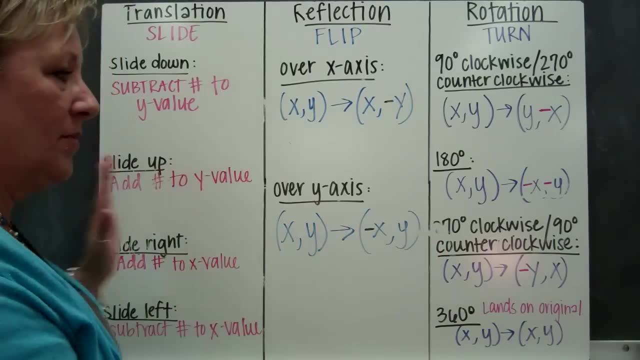 it down, I'm going to subtract from the y value. When I'm sliding it up, I'm going to add to the value. When I'm going to the right, I'm going to add to the x value, and when I'm sliding it to the left, or translating it to the left, I'm going to subtract from. 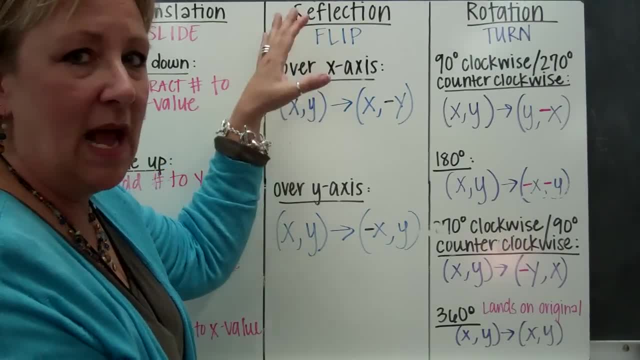 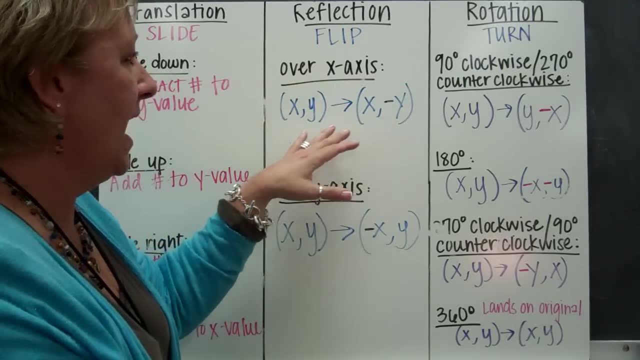 the x axis: S 77, S, 77, S 77, flip it. So you've heard about slide, flip and turn, So I'm going to flip it. So over the x-axis, what happens is my x-y coordinate will become x and a negative y When I'm flipping. 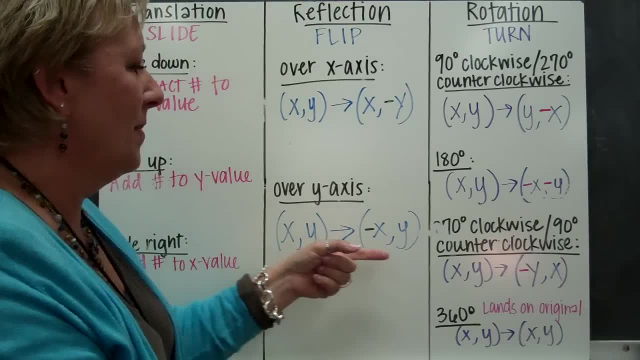 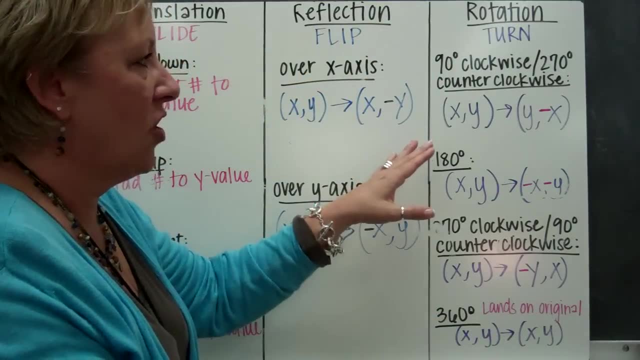 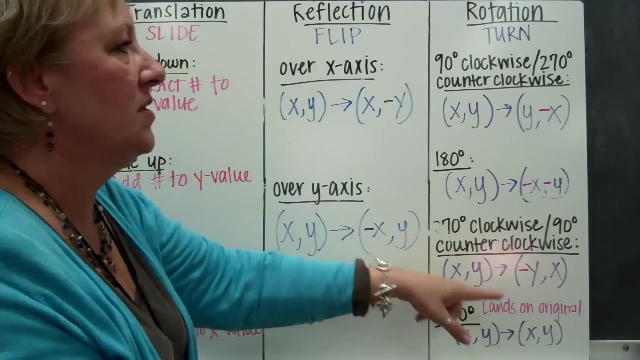 it over the y-axis, my x-y coordinate will become a negative xy. Here the rotations are. where it begins to turn is the hardest one of all. When I'm looking at a 90 degree clockwise or a 270, meaning you're going into the third quadrant, you're going to 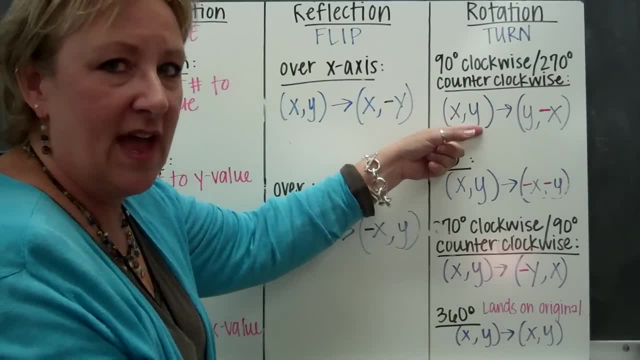 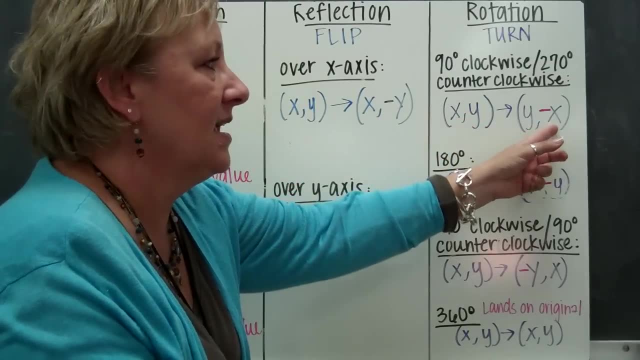 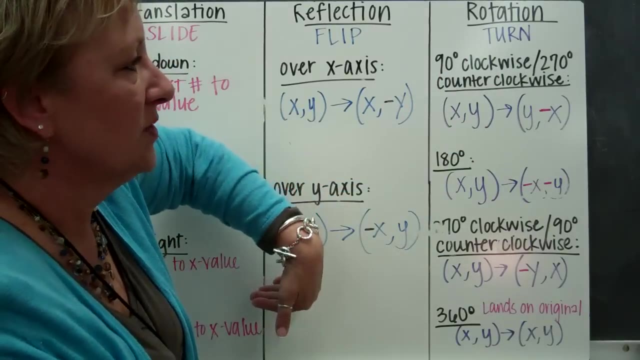 counterclockwise It's going to be your x-y value, which is your image, Your pre-image, will turn into flip the coordinates and make the x value negative. So when I'm going at 90 degrees, just one quadrant or three quadrants, which is going to be 270 degrees, I'm going 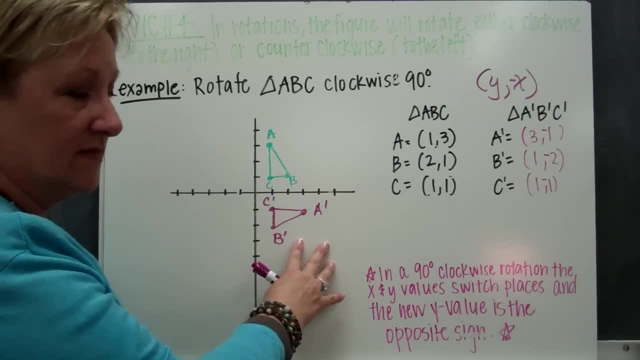 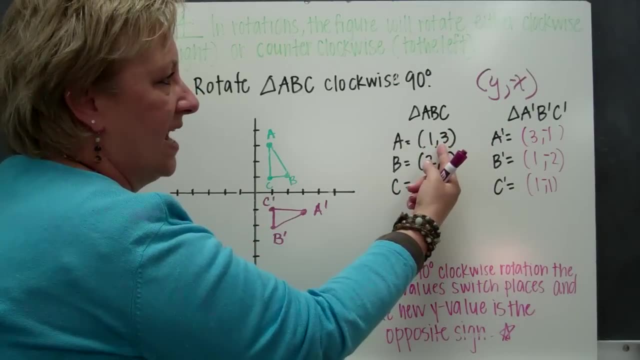 which is going to be quadrant 2, which is going to be positive-negative, Because I have flipped my 2 x's and y's over and I have made my x value, which is now in the y's position, a negative. 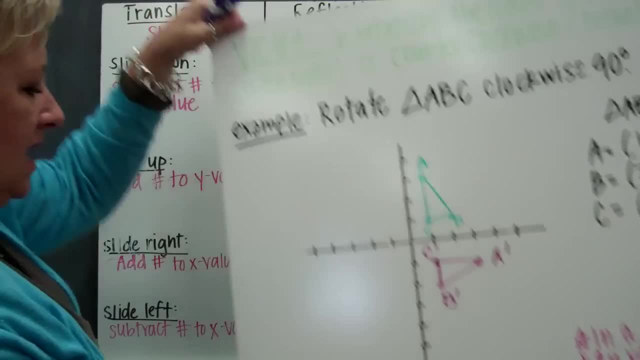 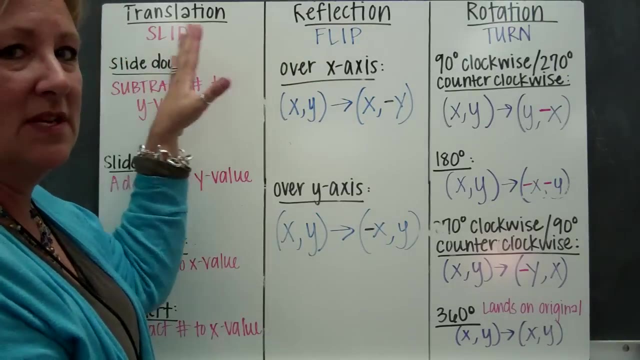 This is just to recap what we've talked about. When we're talking about translations, we're talking about sliding the image either left or right Or up and down. When I'm sliding it down, I'm going to subtract from the y value. 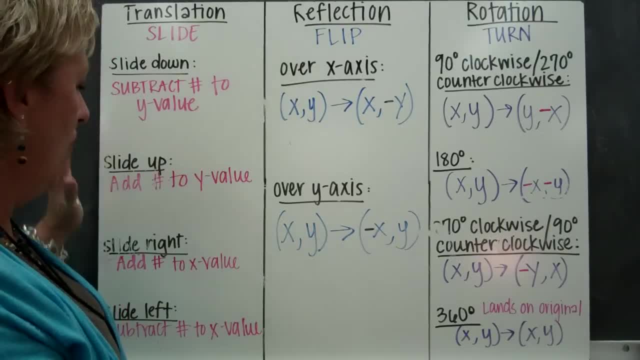 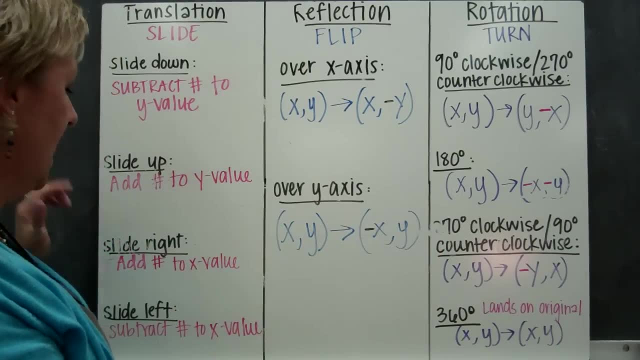 When I'm sliding it up, I'm going to add to the y value. When I'm going to the right, I'm going to add to the x value, And when I'm sliding it to the left or translating it to the left, I'm going to subtract from the x axis. 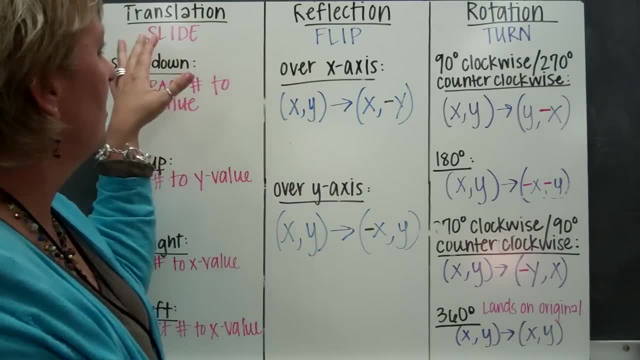 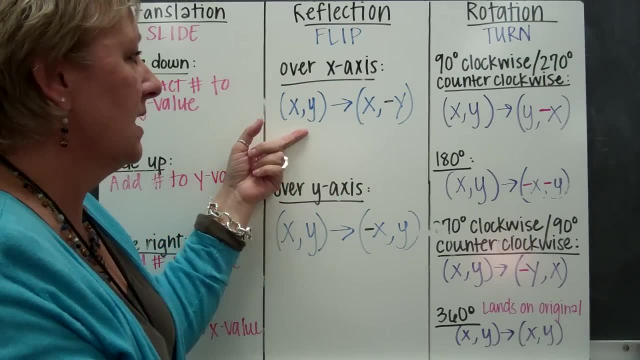 When I'm looking at a reflection, I'm going to flip it. So you've heard about slide, flip and turn, So I'm going to flip it. So, over the x axis, what happens is my x- y coordinate will become x and a negative y. 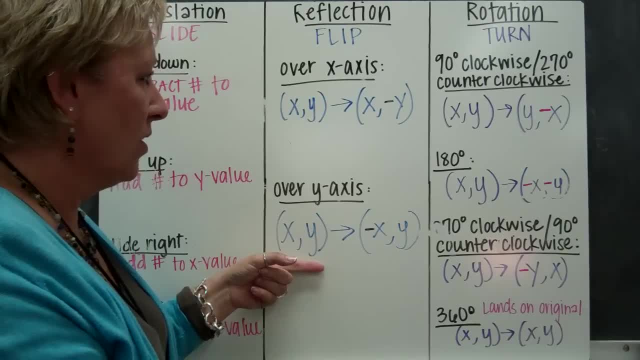 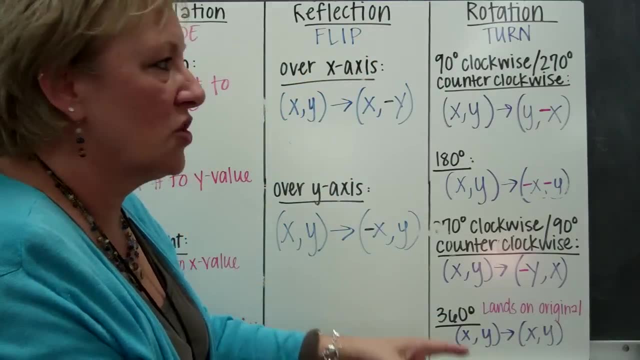 When I'm flipping it over the y axis, my x- y coordinate will become a negative x- y. Here the rotations are. where it begins to turn is the hardest one of all When I'm looking at a 90 degree clockwise or a 270,. 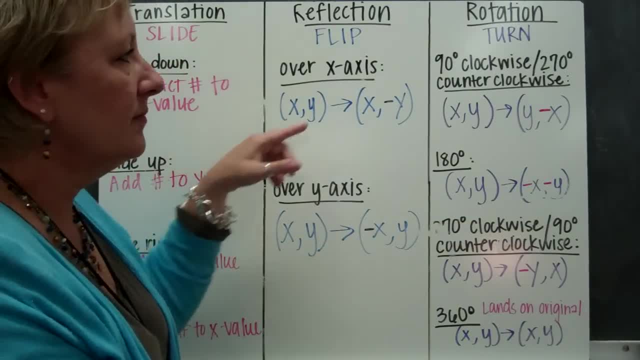 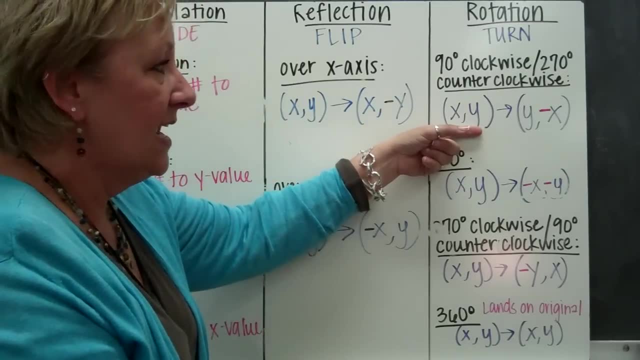 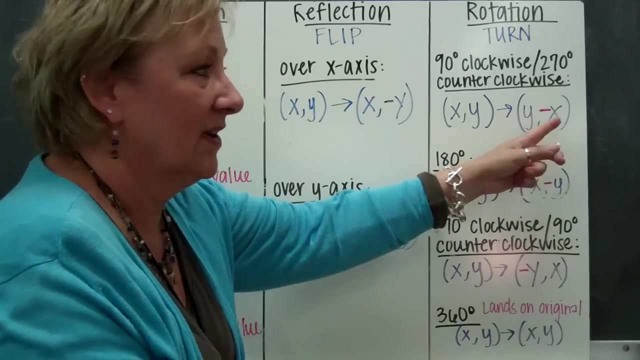 meaning you're going into the third quadrant you're going to counterclockwise is going to be your x- y value, which is your image. your pre-image will turn into flip the coordinates and make the x value negative. So when I'm going at 90 degrees, just one quadrant or three. 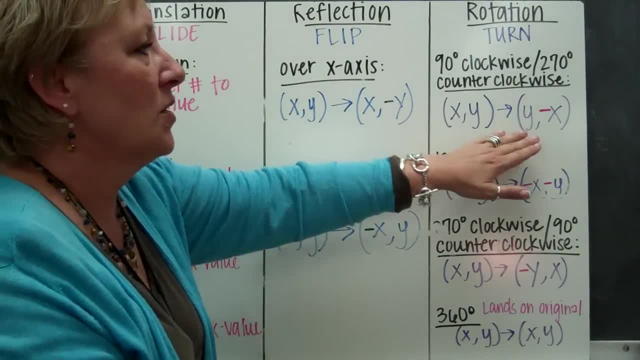 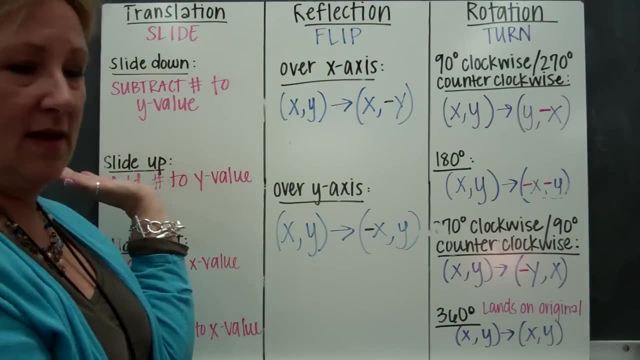 quadrants, which is going to be 270 degrees. I'm going to flip my x and y and make x a negative number. 180 means I'm going from one angle all the way over into a straight line. So my x and y's my pre-image. 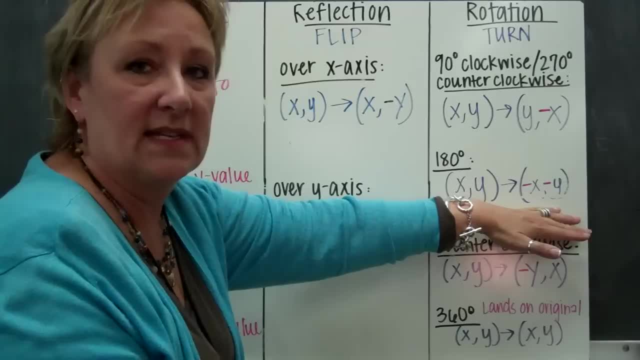 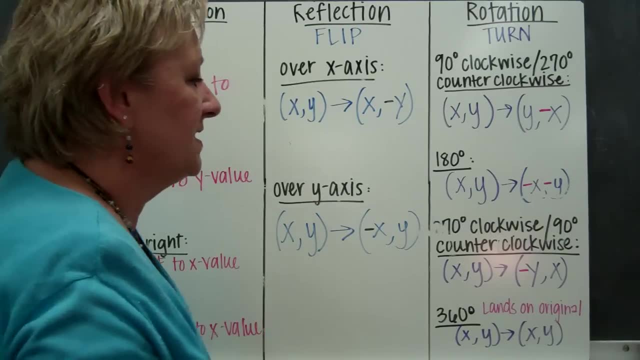 are going to be negative. So I'm going to flip my x and y and make x a negative number. preimage is now going to be: both x and y's are going to be negative or the opposite of each other. For this one, this is going to be 250 degrees. If I'm doing that clockwise. 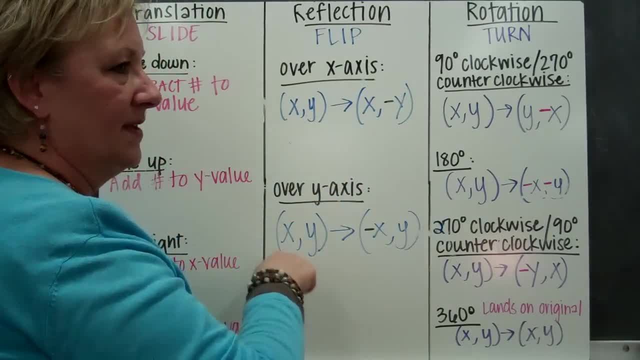 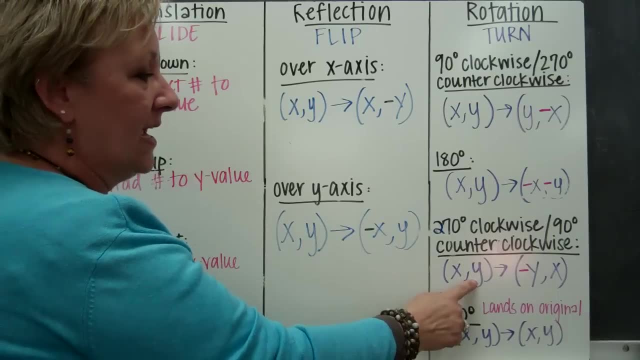 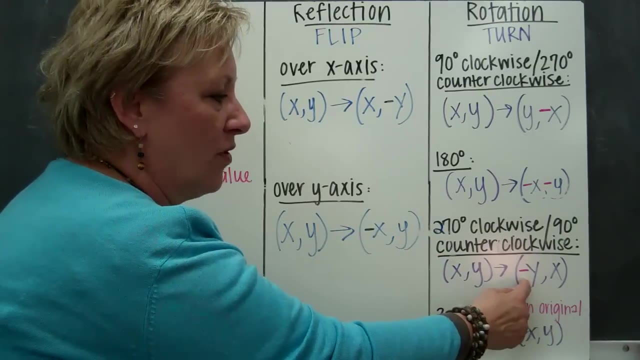 or 950, clockwise meaning around this way, or 90 degrees meaning to the left. I'm going to take my x- y and I'm going to change my x and y's, flip them in the coordinate point and make my y value, or the first one is going to be negative. When I'm going 360, it's going.